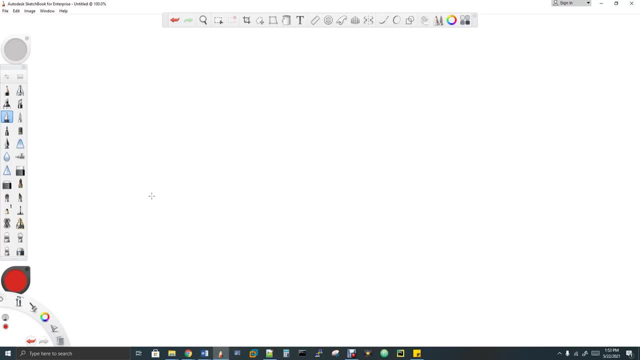 Hi, welcome to Data Engineering. So today we are going to discuss about what is Hive, the introduction of Hive and then the architecture of Hive. And before getting into this video, I have uploaded so many videos for Hadoop, Spark and Hive and so many things. I have given all the 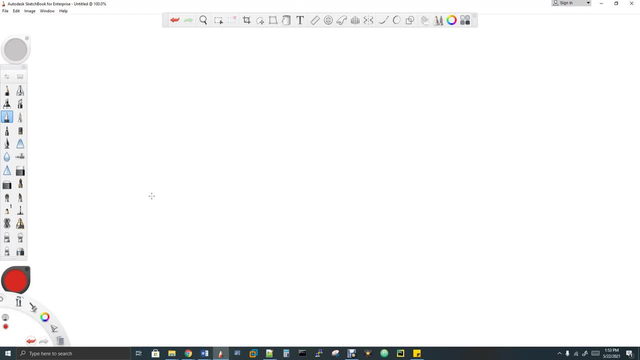 playlist links as a category in my description box, Please, if you want to go through more of my videos, please check those URLs. Okay, let's get into the topic. So Hive. so before getting into Hive, like we need to see a few more things, We will just start with that. So, with respect to 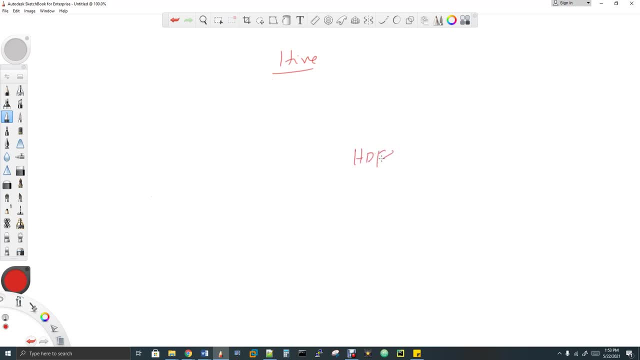 Hadoop. we have two components right. When we say Hadoop, it's combination of HDFS and MapReduce. So that's what Hadoop is right. So HDFS is a place where your data will be distributed and MapReduce is a place where you write jobs, the transformation jobs, and then using Java, and then 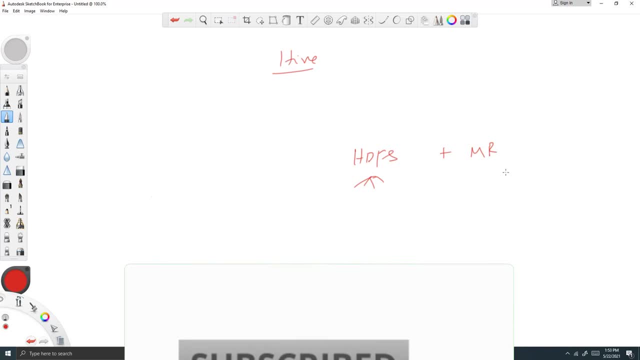 MapReduce will do a distributed processing of your code by reading the data from HDFS. Okay, so now imagine you have to write a join code. So in MapReduce you can't write any sequels. You need to write a Java code. Imagine you are. 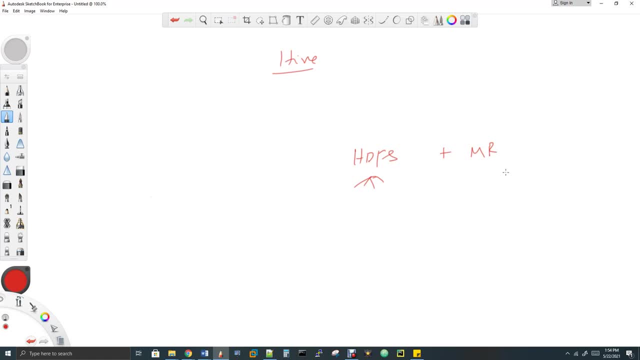 migrating your logics from some other RDBMS database. There is a join query. you have to do which people have been doing in an Oracle. Now you have to do the same in MapReduce. So then you have to write a Java code like 10 to 15 lines of code. you have to write to achieve that. 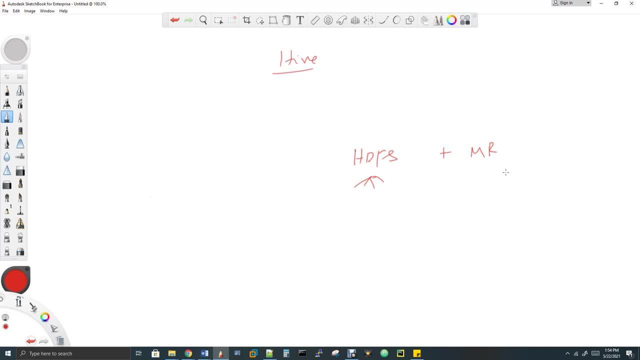 single line SQL join query here. Now here comes the problem. So the SQL developer says: like we are into Hadoop, because MapReduce is really good, It is doing parallel processing and it is distributed parallel processing and the performance is really good. We like all those concepts, But the only problem for us it's always Java. So we need 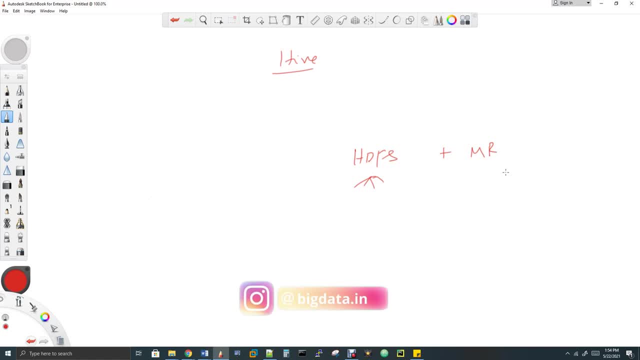 the SQL layer. It will be good, instead of Java, if we have SQL to communicate with MapReduce, And that's where this hive entered into picture. So, if you see, HDFS is the first layer and then you will be having the MapReduce as a core engine for transformation for all doing ETLs extract. 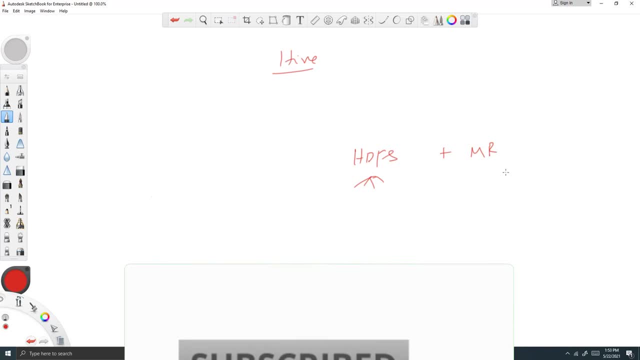 MapReduce will do a distributed processing of your code by reading the data from HDFS. Okay, so now imagine you have to write a join code. So in MapReduce you can't write any sequels. You need to write a Java code. Imagine you are. 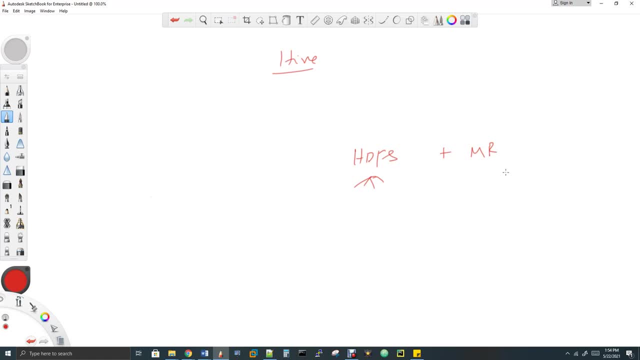 migrating your logics from some other RDBMS database. There is a join query. you have to do which people have been doing in an Oracle. Now you have to do the same in MapReduce. So then you have to write a Java code like 10 to 15 lines of code. you have to write to achieve that. 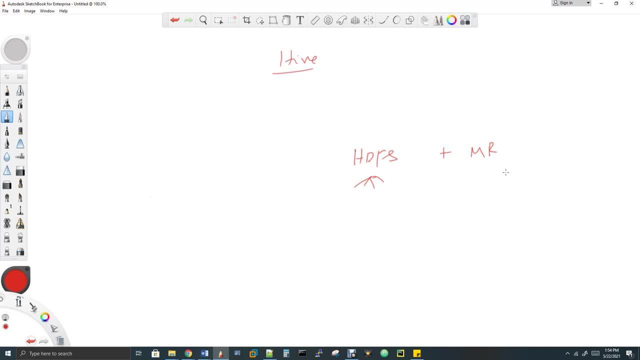 single line SQL join query here. Now here comes the problem. So the SQL developer says: like we are into Hadoop, because MapReduce is really good, It is doing parallel processing and it is distributed parallel processing and the performance is really good. We like all those concepts, But the only problem for us it's always Java. So we need 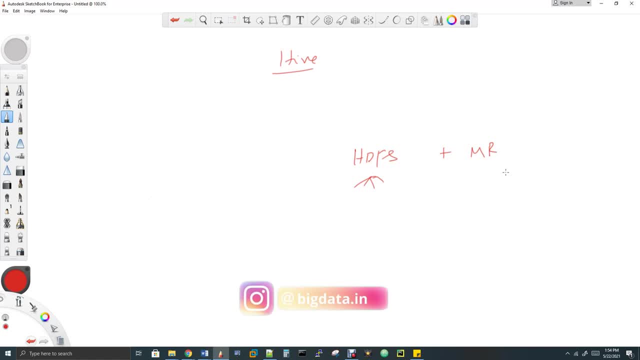 the SQL layer. It will be good, instead of Java, if we have SQL to communicate with MapReduce, And that's where this hive entered into picture. So, if you see, HDFS is the first layer and then you will be having the MapReduce as a core engine for transformation for all doing ETLs extract. 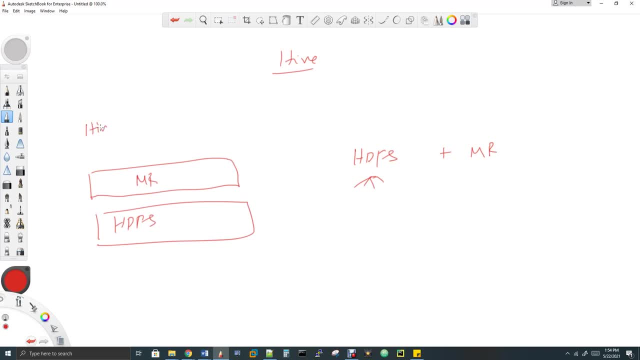 transform Load. So now Hive is invented by Facebook And the language which we use here is SQL. So what Hive is actually? Hive? technically, Hive is a query engine. It's not a database. Very important In real time in projects and with your colleagues, people will always call this Hive as a 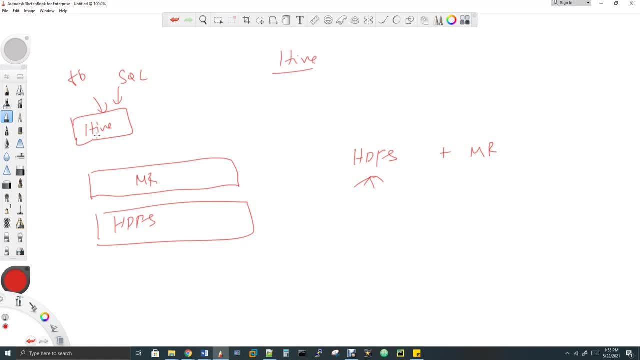 database, But technically speaking, that is a query engine. It's nothing wrong when you say Hive is a database, But since you are in a learning phase, you should understand this. Okay, Hive is a purely a query engine, It's not a database. So here, Hive is a query engine because Hive doesn't. 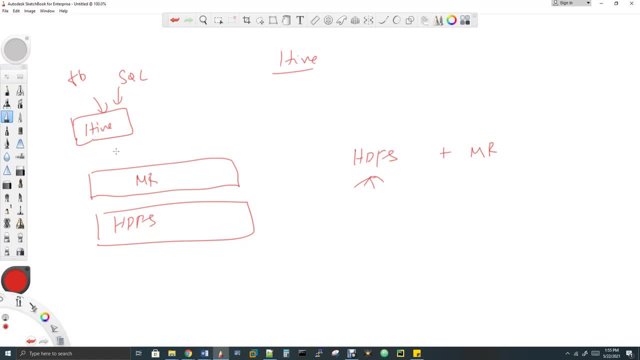 have its own storage to store the data. Hive again, uses HDFS to store the data, And that's the reason. That is also one of the reasons why we are saying Hive is not a DB, Whereas if you go for Oracle or MySQL it has its own storage Come query engine, Okay. So here Facebook invented 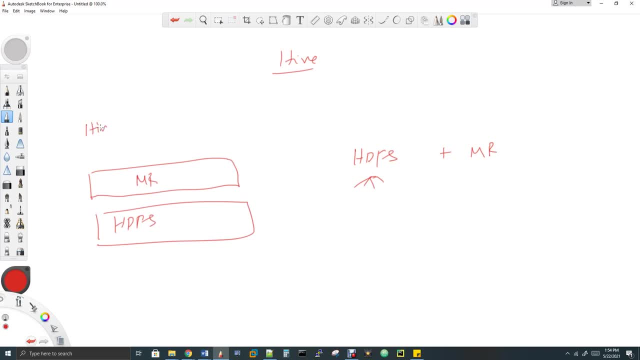 transform Load. So now Hive is invented by Facebook And the language which we use here is SQL. So what Hive is actually? Hive? technically, Hive is a query engine. It's not a database. Very important In real time in projects and with your colleagues, people will always call this Hive as a 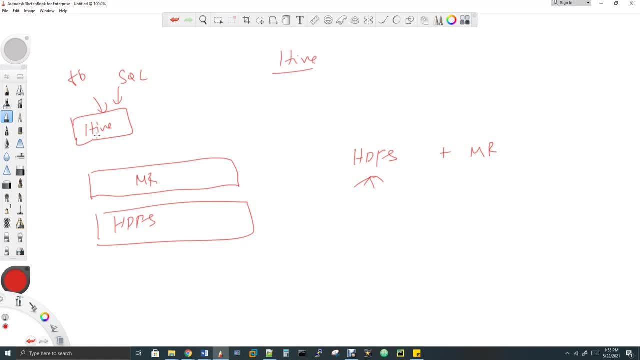 database, But technically speaking, that is a query engine. It's nothing wrong when you say Hive is a database, But since you are in a learning phase, you should understand this. Okay, Hive is a purely a query engine, It's not a database. So here, Hive is a query engine because Hive doesn't. 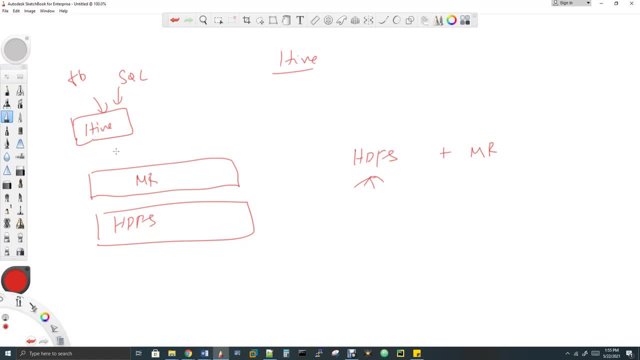 have its own storage to store the data. Hive again, uses HDFS to store the data, And that's the reason. That is also one of the reasons why we are saying Hive is not a DB, Whereas if you go for Oracle or MySQL it has its own storage Come query engine, Okay. So here Facebook invented 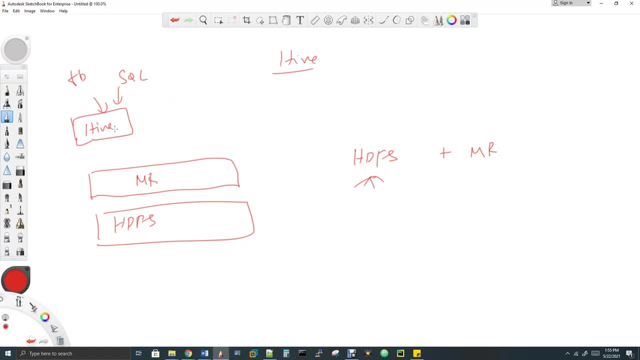 this Hive and it is an open source. It's available in Apache. You can download and install it in your machine. So the prerequisite to get into Hive is you need to know HDFS basic of MapReduce and SQL queries. When I say SQL queries, no complex queries like stored procedure or trigger, That kind of SQL. 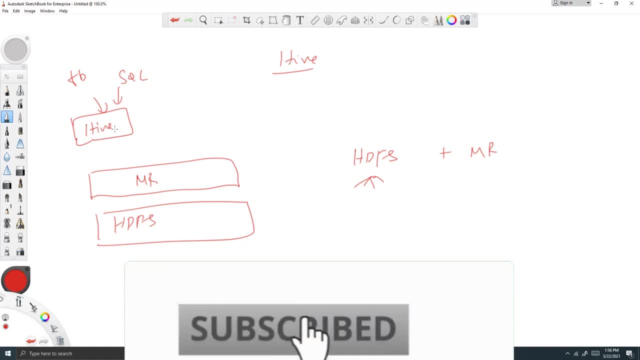 knowledge is not required. Create, update, delete, insert, select sub queries and joins is wide enough for you to get into Hive. These are all the prerequisites. Now Hive acts as a vehicle which again runs on the engine MapReduce. That's very important to understand And that's why we 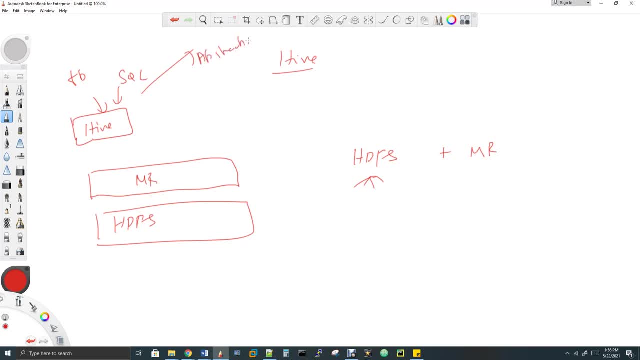 call Hive is abstraction of MapReduce. We call Hive as abstraction of MapReduce, So Hive internally use MapReduce engine to process the query. So instead of Java I'm going to communicate with SQL, So I want to write a Java code. So just. 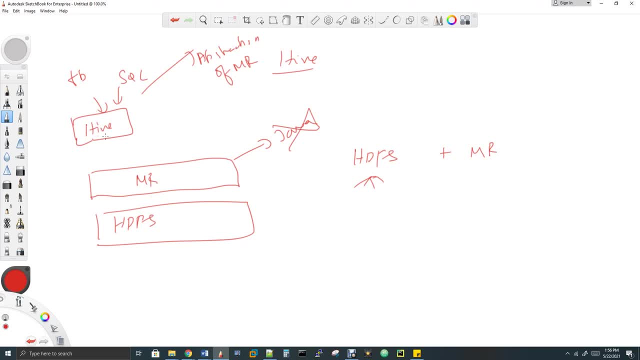 bypassing this with SQL via Hive. Okay, Hive just replaced the Java part, It's not replacing the MapReduce. That's very important. People used to say like that. People used to say: I'm not using MapReduce, I'm using Hive. No, you have to correct the statement. You are using SQL, You are using. 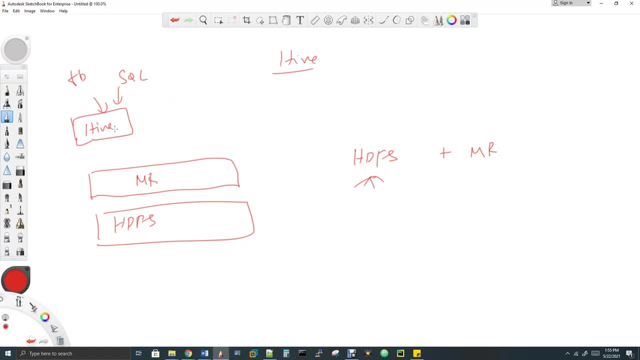 this Hive and it is an open source. It's available in Apache. You can download and install it in your machine. So the prerequisite to get into Hive is you need to know HDFS basic of MapReduce and SQL queries. When I say SQL queries, no complex queries like stored procedure or trigger, That kind of SQL. 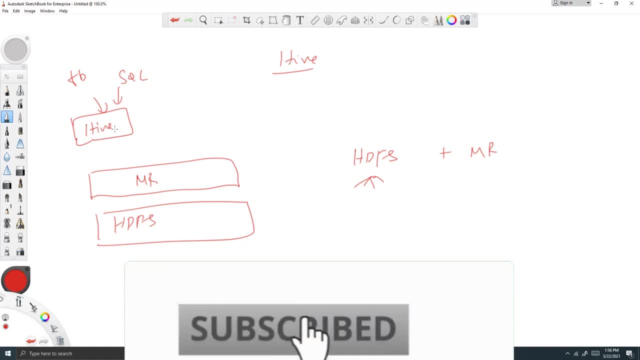 knowledge is not required. Create, update, delete, insert, select sub queries and joins is wide enough for you to get into Hive. These are all the prerequisites. Now Hive acts as a vehicle which again runs on the engine MapReduce. That's very important to understand And that's why we 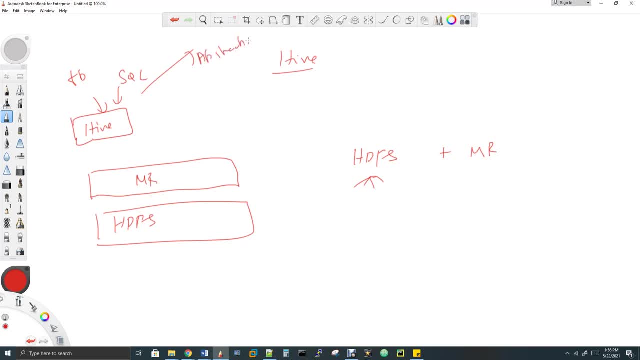 call Hive is abstraction of MapReduce. We call Hive as abstraction of MapReduce, So Hive internally use MapReduce engine to process the query. So instead of Java I'm going to communicate with SQL, So I want to write a Java code. So just. 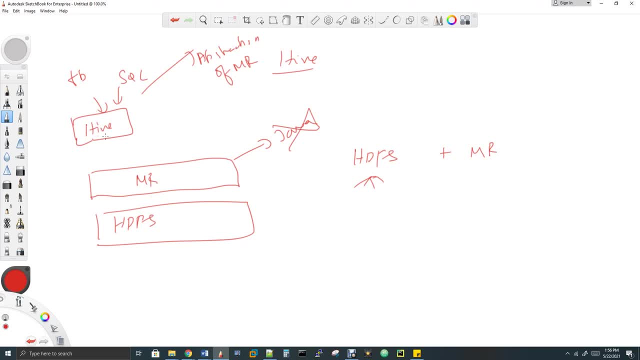 bypassing this with SQL via Hive. Okay, Hive just replaced the Java part, It's not replacing the MapReduce. That's very important. People used to say like that. People used to say: I'm not using MapReduce, I'm using Hive. No, you have to correct the statement. You are using SQL, You are using. 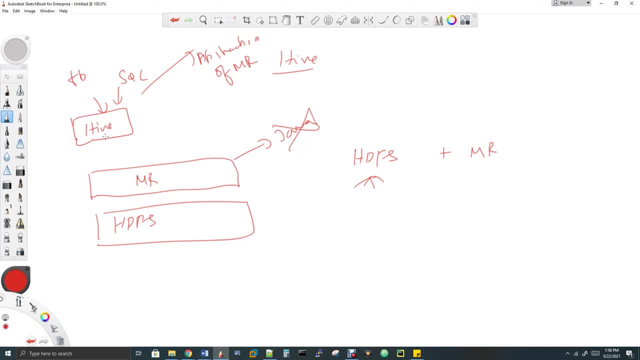 Hive And you are not using Java. That is what you have to say. So when you say that you are not using MapReduce, then I will think: then instead of MapReduce, you are using some other engine to run Hive. That's how I will think. So that's a wrong thing. So you are using MapReduce, but you are. 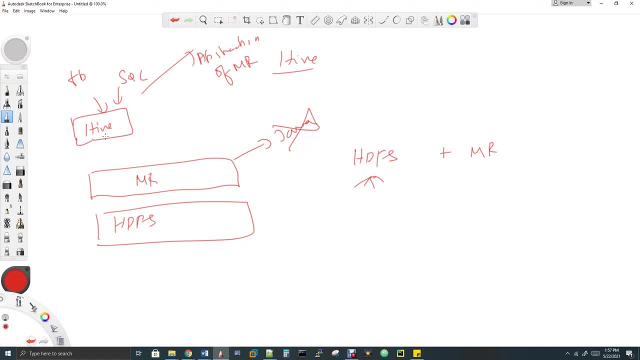 using SQL instead of Java via Hive. Fine, So now what Hive will do? Hive, like it again, reads the data from HDFS and then process it in Hive with the help of MapReduce, And then the output can be stored again back to HDFS. Okay, 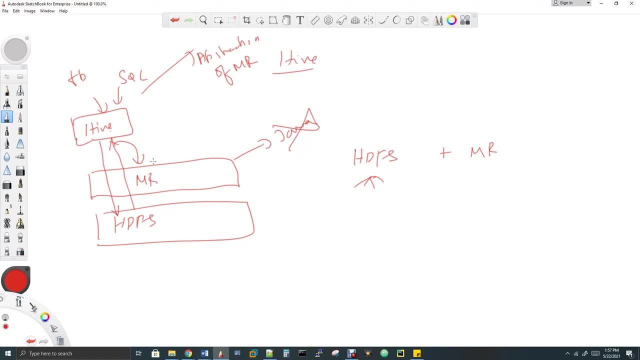 Now we understood where exactly this Hive comes into picture and what is Hive and who developed it. Okay, This is what we have seen Now, like we will get more into the Hive internals and the architecture, So before getting into that. so we have similar to MapReduce. we have one more. 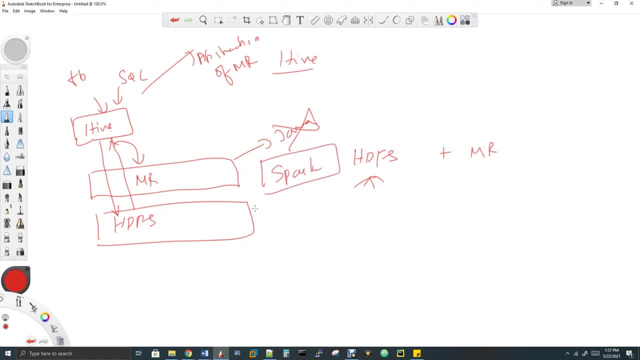 engine right called Spark right. So Spark is replacement of MapReduce. It's not replacement of the entire Hadoop. That's very important. I have saying this in many videos. I will still use to say that. So Spark just replaced the MapReduce, but not the whole. 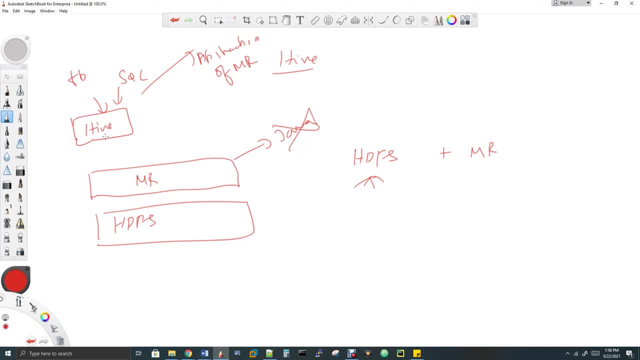 Hive And you are not using Java. That is what you have to say. So when you say that you are not using MapReduce, then I will think: then instead of MapReduce, you are using some other engine to run Hive. That's how I will think. So that's a wrong thing. So you are using MapReduce, but you are. 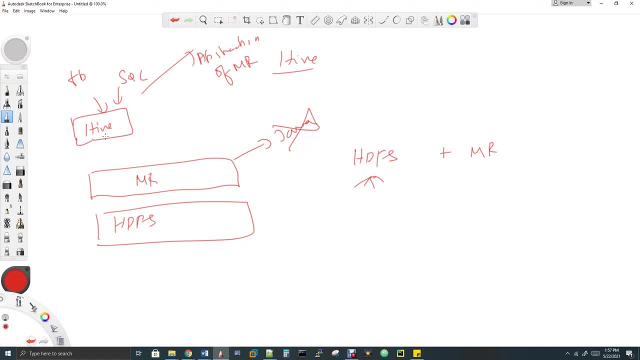 using SQL instead of Java via Hive. Fine, So now what Hive will do? Hive, like it again, reads the data from HDFS and then process it in Hive with the help of MapReduce, And then the output can be stored again back to HDFS. Okay, 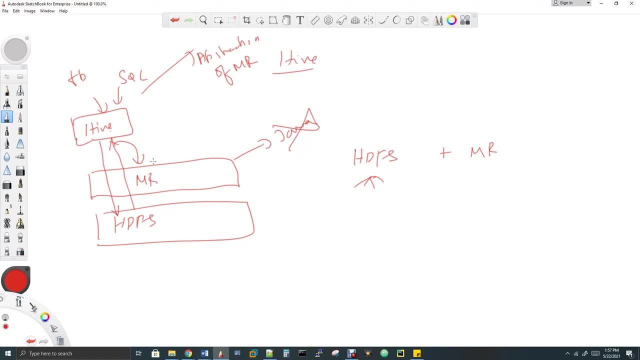 Now we understood where exactly this Hive comes into picture and what is Hive and who developed it. Okay, This is what we have seen Now, like we will get more into the Hive internals and the architecture, So before getting into that. so we have similar to MapReduce. we have one more. 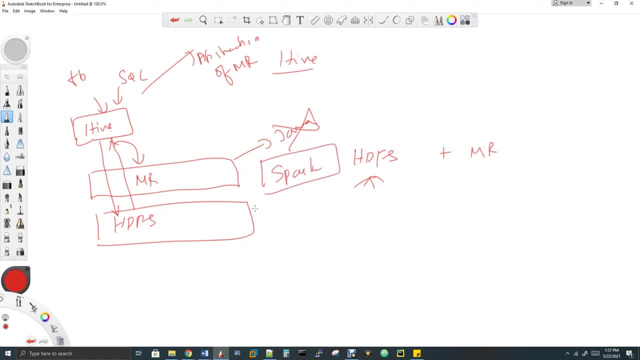 engine right called Spark right. So Spark is replacement of MapReduce. It's not replacement of the entire Hadoop. That's very important. I have saying this in many videos. I will still use to say that. So Spark just replaced the MapReduce, but not the whole. 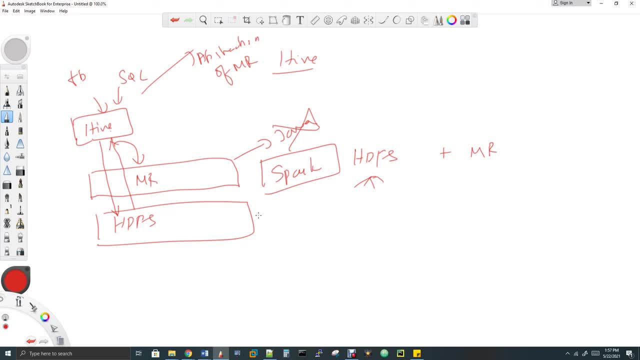 Hadoop framework. So why I'm telling this here? right? So Hive can also run on Spark engine instead of MapReduce. Okay, So Hive is a vehicle, So you have MapReduce engine which operates the vehicle. Now you remove MapReduce and you are changing your engine to Spark, So your same. 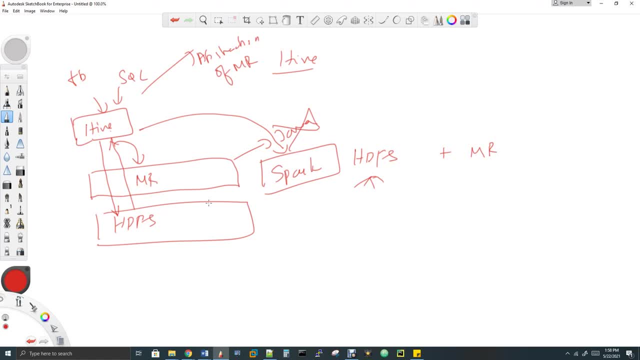 Hive vehicle will run more faster. So that is how it is. Okay Now, so you can ask me another question. So that means I don't want to go for Spark and MapReduce To write a code. you mean to say, we can do everything in SQL itself. Okay, So you can't. 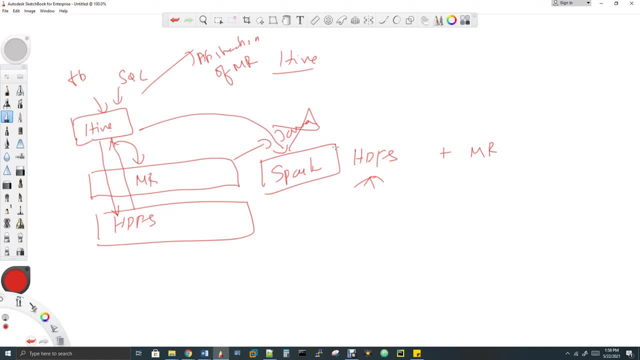 do everything in SQL. There will be some complex processing transformations you have to do which is not compatible with Hive. Then you have to go for Spark and writing programs or MapReduce to write the programs. But Hive is more matured in recent days So you can. 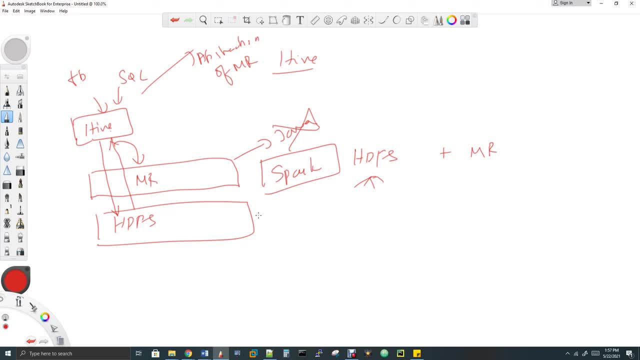 Hadoop framework. So why I'm telling this here? right? So Hive can also run on Spark engine instead of MapReduce. Okay, So Hive is a vehicle, So you have MapReduce engine which operates the vehicle. Now you remove MapReduce and you are changing your engine to Spark, So your same. 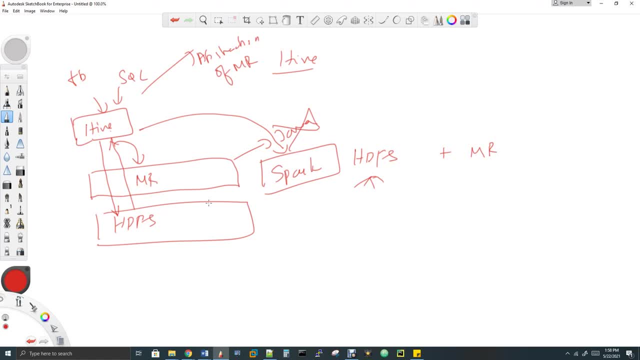 Hive vehicle will run more faster. So that is how it is. Okay Now, so you can ask me another question. So that means I don't want to go for Spark and MapReduce To write a code. you mean to say, we can do everything in SQL itself. Okay, So you can't. 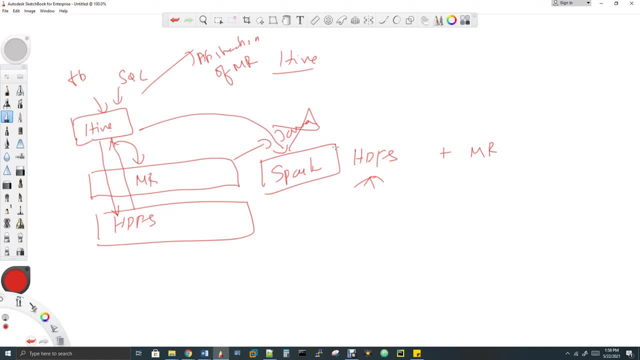 do everything in SQL. There will be some complex processing transformations you have to do which is not compatible with Hive. Then you have to go for Spark and writing programs or MapReduce to write the programs. But Hive is more matured in recent days So you can. 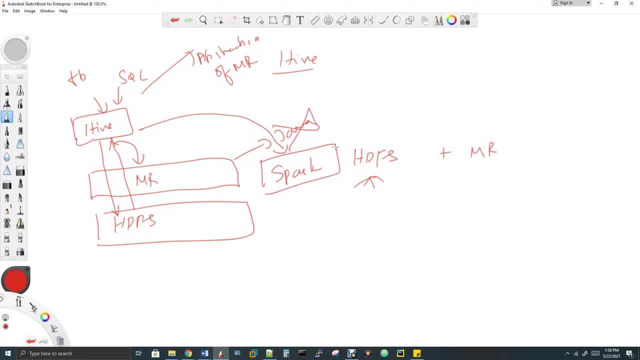 do so many things in Hive itself, but still some things for some extra performance and some extra optimization and some extra complex logics. If there is a condition, then you have to go for directly to the Hive So you can do everything in SQL itself. So you can. 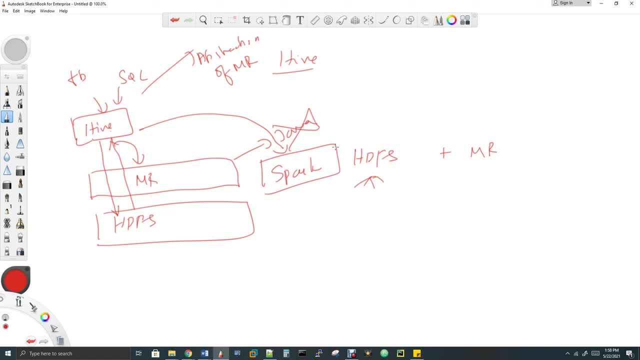 do MapReduce and Spark to write in the programs instead of doing in Hive queries? Okay Fine. So now we get into the next level of understanding the Hive internals. Okay Fine, So here how Hive works. when there is a request, response happens. Now imagine I installed my Hive. 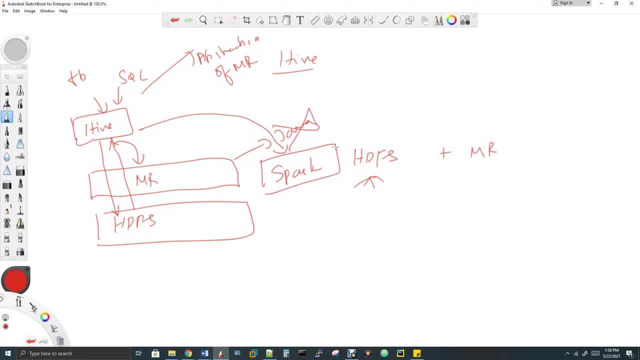 do so many things in Hive itself, but still some things for some extra performance and some extra optimization and some extra complex logics. If there is a condition, then you have to go for directly to the Hive So you can do everything in SQL itself. So you can. 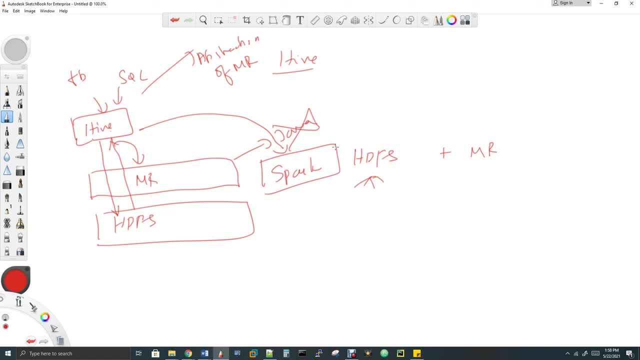 do MapReduce and Spark to write in the programs instead of doing in Hive queries? Okay Fine. So now we get into the next level of understanding the Hive internals. Okay Fine, So here how Hive works. when there is a request, response happens. Now imagine I installed my Hive. 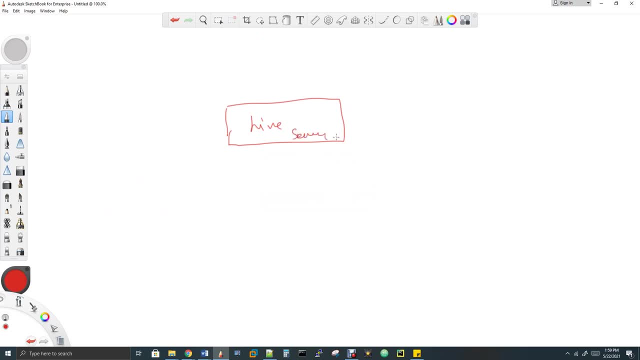 Okay, So whenever you install an Hive, there will be a server running. Okay, Now you are sending a request. So the request is through CLI command line interface, That means in the terminal. if you run bin slash Hive, Hive will be get started like this: where you can. 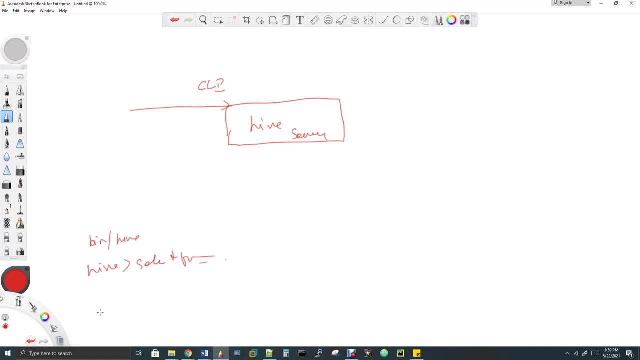 run all your queries. select star from, et cetera. Okay, CLI command line interface. Okay, So now the request. what I'm sending via CLI is create table test. Okay, So the request goes to my Hive server. So now, what Hive server will do So when I create a table? so Hive. 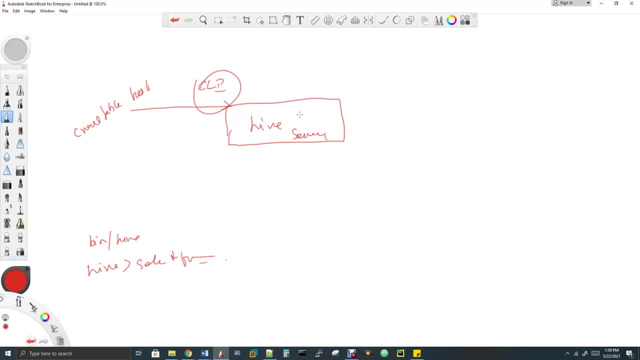 has a metadata. Okay, What? what that metadata has? the metadata will have all the all the Hive table information, but not the data. That's very important. So metadata of Hive will store all the table information. Table information means how many columns it has. 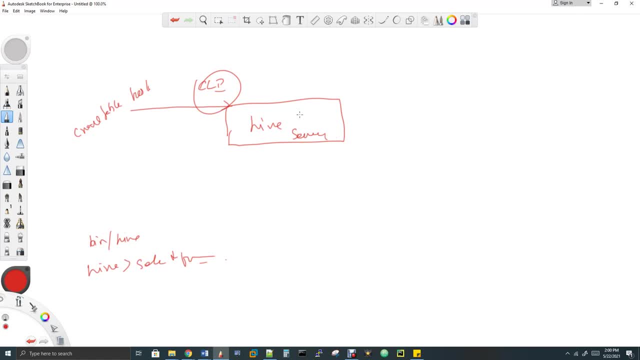 whether it has an index or not in the table. So those kinds of information. So the Hive metadata is different from the metadata what maintains in the name node. Okay, They are different. Okay, Now, where this Hive metadata will get stored. Important point: This is: 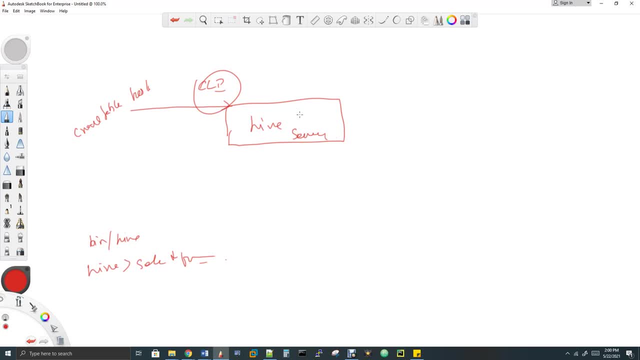 in most asked the question in interviews. also, And even for your self-understanding, this is very important. Hive will store the metadata in a RDBMS database only. That's very important. So Hive will store the metadata information in an RDBMS. It can be Oracle or it can be DB2.. It can. 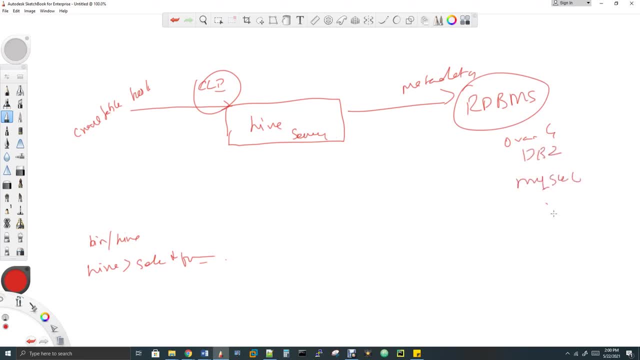 be MySQL or any RDBMS. Even if you see there is an installation video of Hive, it's there in my playlist link you can find below. I have shown you the installation of Hive with MySQL. So where Hive use MySQL to store the metadata. 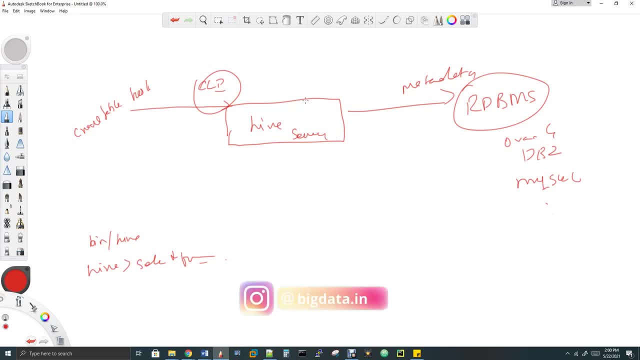 And very important thing, Hive uses this RDBMS to store only the metadata, but not the data that you insert. That is very important. The data that you insert will store only in HDFS, So the only reason we use RDBMS here is to store the metadata information of Hive. Very 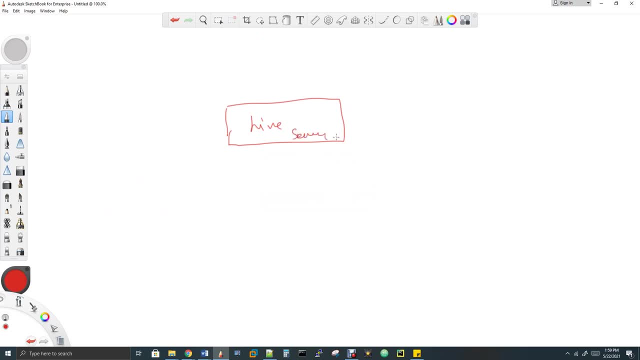 Okay, So whenever you install an Hive, there will be a server running. Okay, Now you are sending a request. So the request is through CLI command line interface, That means in the terminal. if you run bin slash Hive, Hive will be get started like this: where you can. 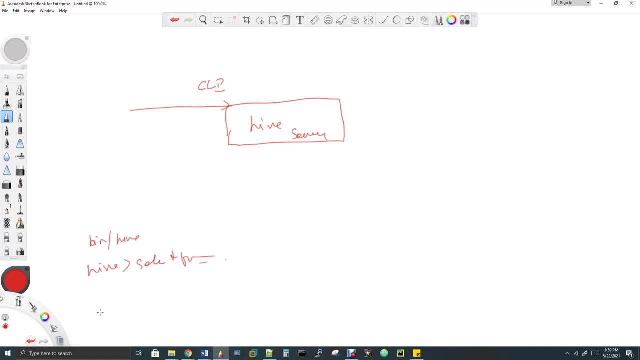 run all your queries. select star from, et cetera. Okay, CLI command line interface. Okay, So now the request. what I'm sending via CLI is create table test. Okay, So the request goes to my Hive server. So now, what Hive server will do So when I create a table? so Hive. 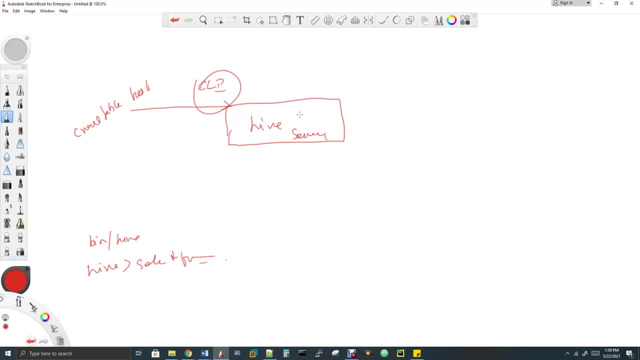 has a metadata. Okay, What? what that metadata has? the metadata will have all the all the Hive table information, but not the data. That's very important. So metadata of Hive will store all the table information. Table information means how many columns it has. 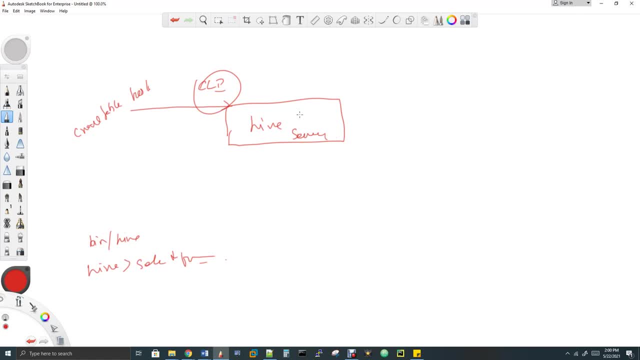 whether it has an index or not in the table. So those kinds of information. So the Hive metadata is different from the metadata what maintains in the name node. Okay, They are different. Okay, Now, where this Hive metadata will get stored. Important point: This is: 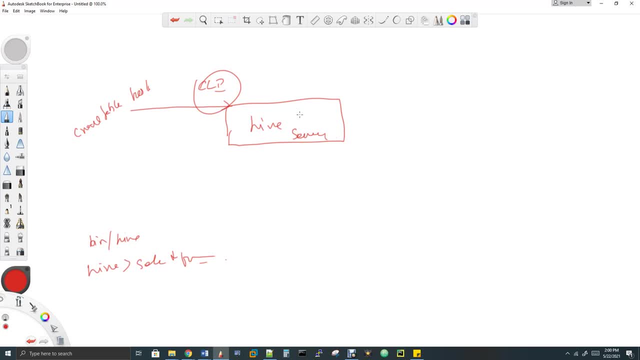 in most asked the question in interviews. also, And even for your self-understanding, this is very important. Hive will store the metadata in a RDBMS database only. That's very important. So Hive will store the metadata information in an RDBMS. It can be Oracle or it can be DB2.. It can. 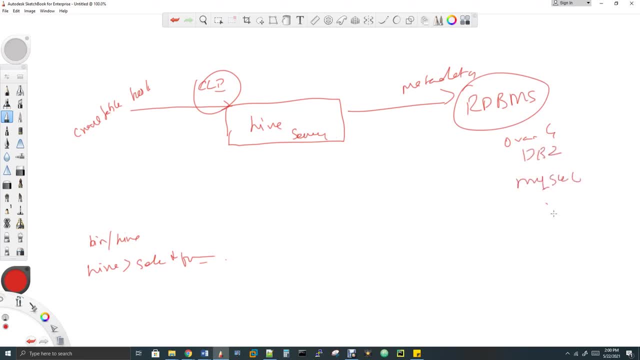 be MySQL or any RDBMS. Even if you see there is an installation video of Hive, it's there in my playlist link you can find below. I have shown you the installation of Hive with MySQL. So where Hive use MySQL to store the metadata. 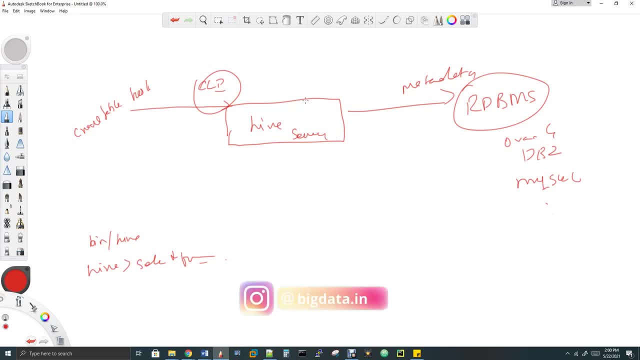 And very important thing, Hive uses this RDBMS to store only the metadata, but not the data that you insert. That is very important. The data that you insert will store only in HDFS, So the only reason we use RDBMS here is to store the metadata information of Hive. Very 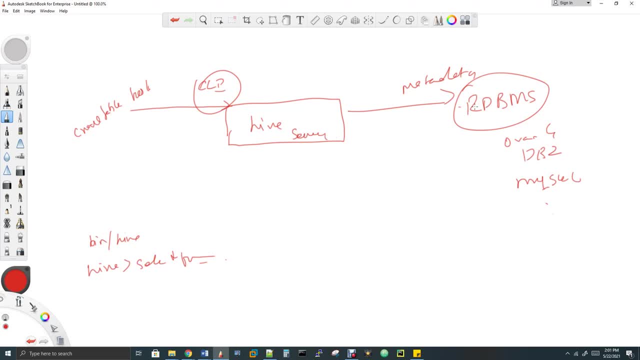 important to understand because when people used to think, when they learn it in the beginning stage, they think that metadata is where, like Hive, data also will get stored. No, it won't. If you see, in Oracle They will store metadata for MySQL and all The metadata also will be stored inside Oracle. 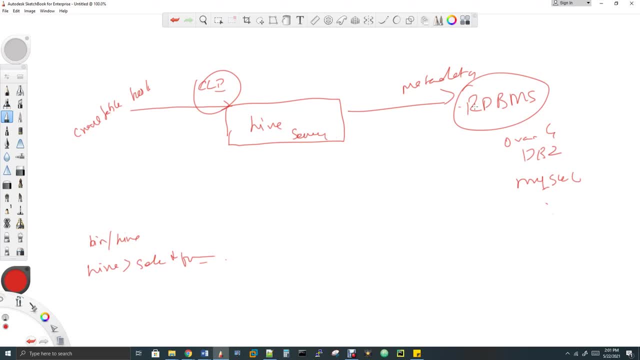 inside MySQL itself, But in Hive alone. they are decoupling the metadata part. The metadata will be stored in a different place, That is RDBMS. Now you created the table Again through CLA. I am sending in another request to insert. 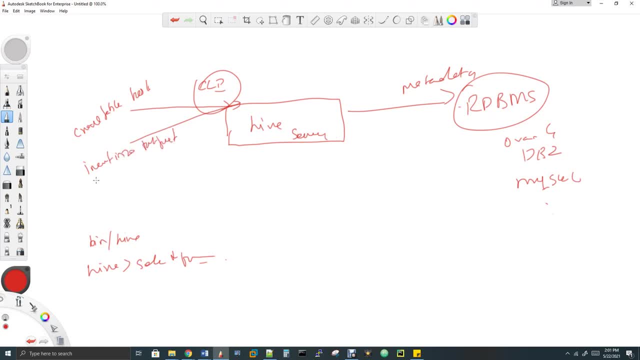 Insert into table Test. So now I am inserting a data or you can use a loadData. So loadData command is to load the data in bulk as a file to a table. Insert means 1 by 1.. So now this request comes, what i will do? it will get the metadata information, like this table test, and 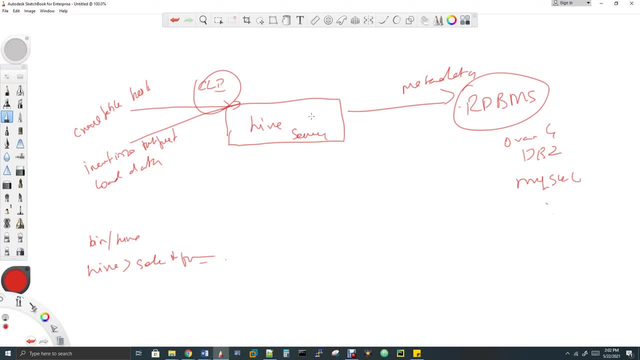 how many columns it has and all those information and based on that schema information, i will store the data as a table in your hdfs. okay, so again, the data will get stored in hdfs only. okay with the, with the, with all those row column matchings with schema will happen. that's how you will. 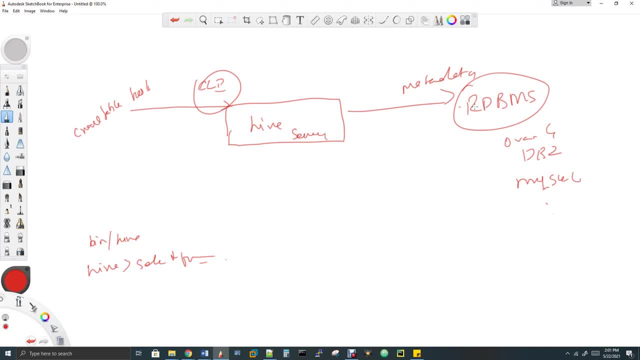 important to understand because when people used to think, when they learn it in the beginning stage, they think that metadata is where, like Hive, data also will get stored. No, it won't. If you see in Oracle, If you see in MySQL, and all the metadata also will be stored inside Oracle, inside MySQL. 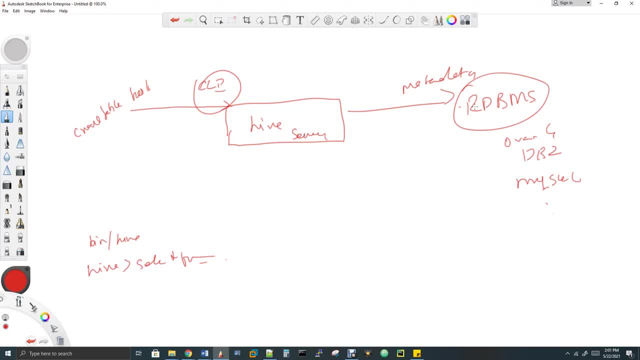 itself, But in Hive alone. like they are decoupling that metadata part, The metadata will get stored in a different place. That is RDBMS. Now you created the table. Now again through CLI, I am sending in another request to insert. 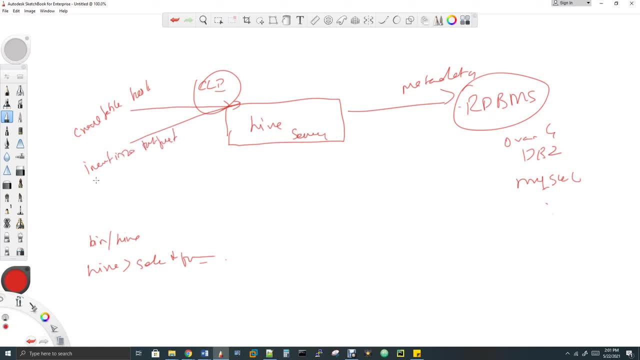 Insert into table test. So now I am inserting a data or you can use a load data. So load data command is to load the data in bulk as a file to a table. Insert means one by one request comes what i will do. it will get the metadata information, like this table test, and 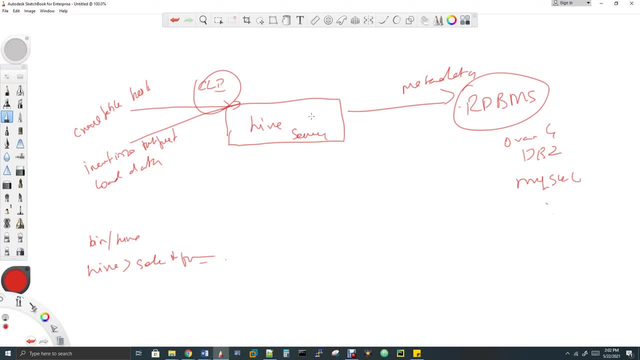 how many columns it has and all those information and based on that schema information, i will store the data as a table in your hdfs. okay, so again, the data will get stored in hdfs only. okay with the, with the, with all those row column matchings with schema will happen. that's how you will. 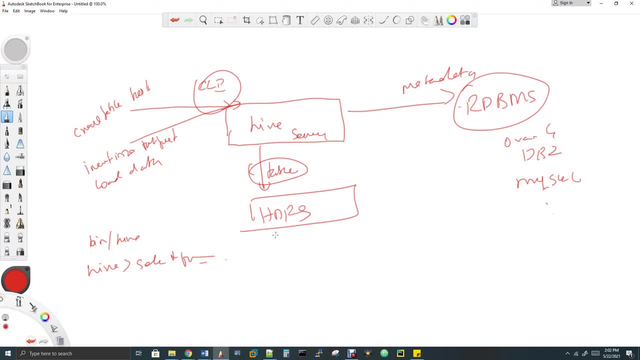 maintain as a metadata in rdbms, but data gets stored in hdfs. now i'm sending a select query to read this inserted data. so select star from test. now what happens? right? so this particular query. so it goes to hive server. first the first, this query, uh, first after getting this query as 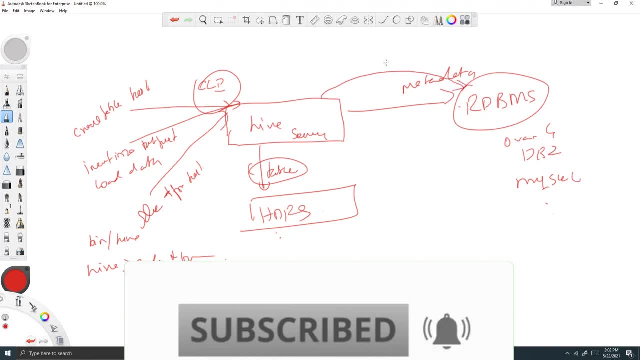 a request. what i will do. it will first query the metadata information and then it will get the data from hdfs and then it will show you in a row. so i will show you in a row, column view. so this is what happens when you do a. 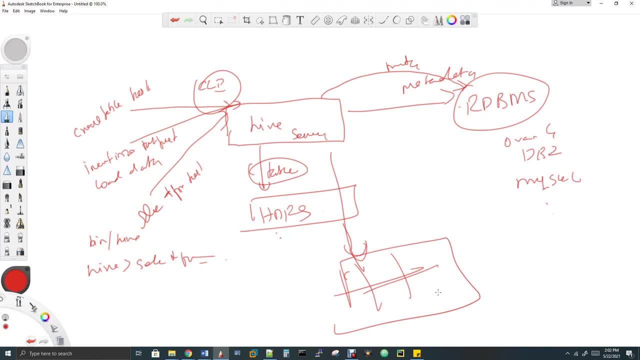 request. so create request, insert request and select request. this is what happened. so whenever you send a request for select, hive will query the metadata, the table information and with that, the data, what you have inserted. it will match and it will show you as a table. so this is what. 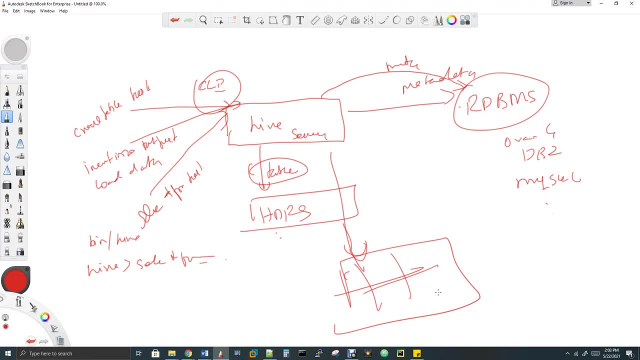 happens every time. okay, so rdbms is why they are storing metadata in. rdbms is a design. that's how it gets stored. because they don't want to have it within the hive itself, they decouple to the metadata storage part outside the world of. 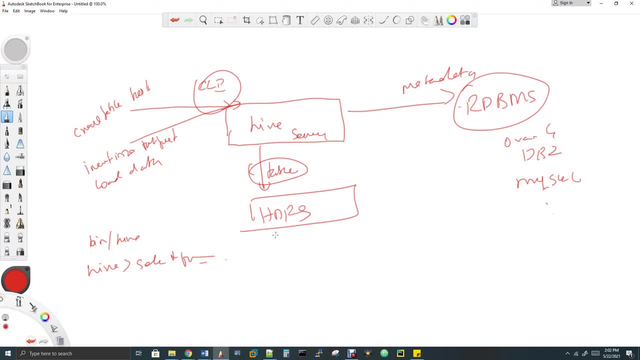 maintain as a metadata in rdbms, but data gets stored in hdfs. now i'm sending a select query to read this inserted data. so select star from test. now what happens? right? so this particular query. so it goes to hive server. first the first, this query, uh, first after getting this query as 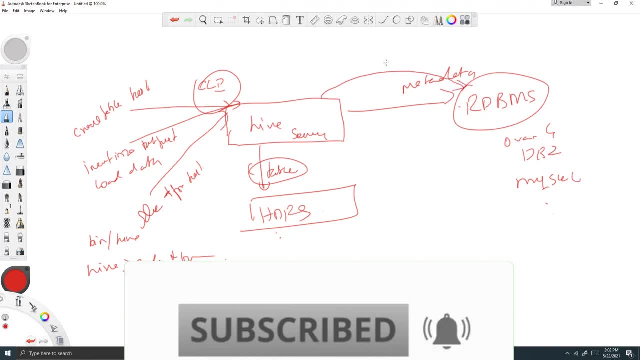 a request. what i will do. it will first query the metadata information and then it will get the data from hdfs and then it will show you in a row. so i will show you in a row, column view. so this is what happens when you do a. 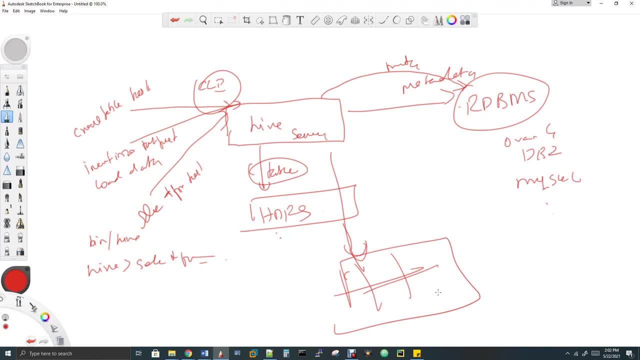 request. so create request, insert request and select request. this is what happened. so whenever you send a request for select, hive will query the metadata, the table information and with that, the data, what you have inserted. it will match and it will show you as a table. so this is what. 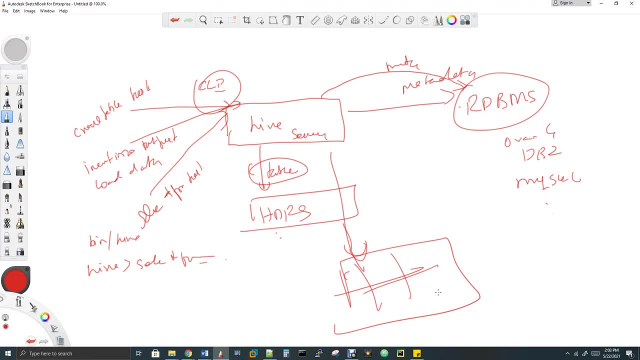 happens every time. okay, so rdbms is why they are storing metadata in. rdbms is a design. that's how it gets stored. because they don't want to have it within the hive itself, they decouple to the metadata storage part outside the world of. 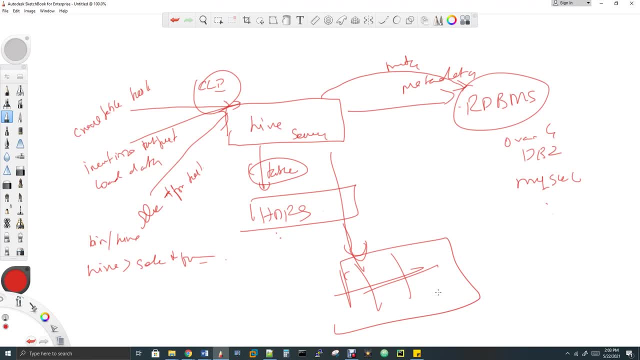 hive. okay. so now i'm going to tell you one more thing. now, imagine i'm not installing rdbms in hive. i mean, while installing hive, you should install rdbms also, so that's when you will store your metadata in a different database. right now there is a case like: imagine you don't want to install. 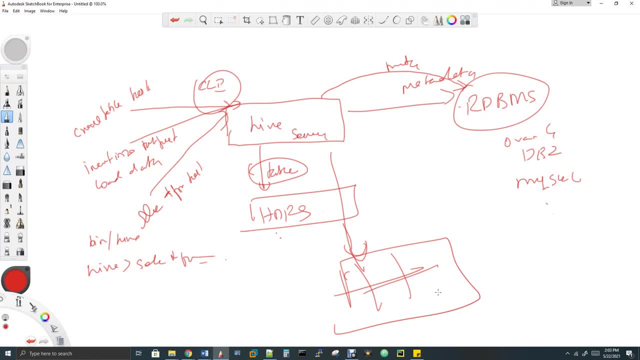 rdbms, just go to apache hive site and download the hive. and you don't want to install rdbms, just install hive only. in that case how the metadata will be get stored. so that is a question here. so what i said to you- you don't want to install rdbms, just install hive only- is enough. so in that, 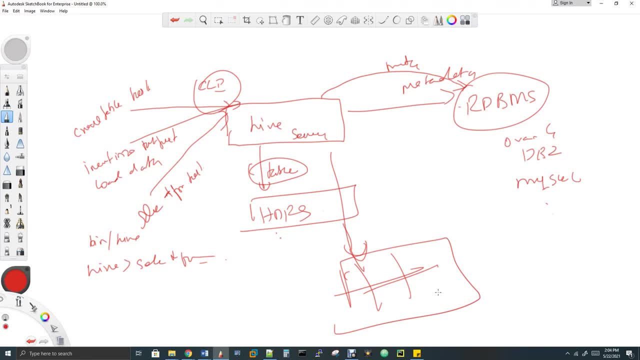 case where the metadata will store. i will tell you that. so you install hive only. okay, i will just go here. so whenever you download hive, right, you installed hive. so when there is no separate rdbms available in your, in your installation, in your machine, then what hive will do? hive itself will. 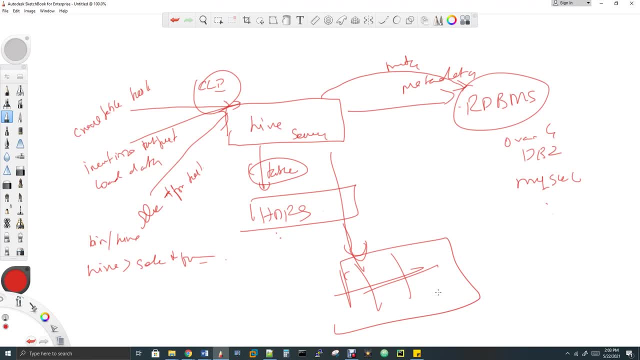 hive. okay. so now i'm going to tell you one more thing. now, imagine i'm not installing rdbms in hive. i mean, while installing hive, you should install rdbms also, so that's when you will store your metadata in a different database. right now there is a case like: imagine you don't want to install. 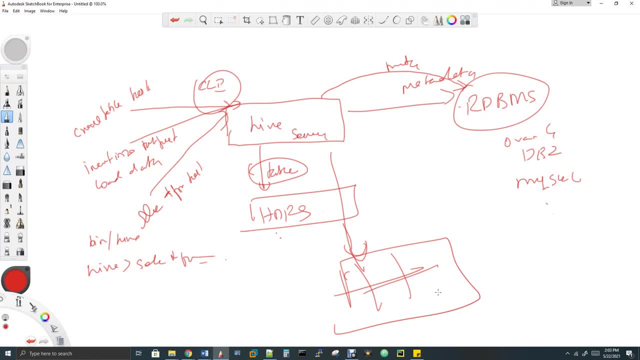 rdbms, just go to apache hive site and download the hive. and you don't want to install rdbms, just install hive only. in that case how the metadata will be get stored. so that is a question here. so what i said to you- you don't want to install rdbms, just install hive only- is enough. so in that, 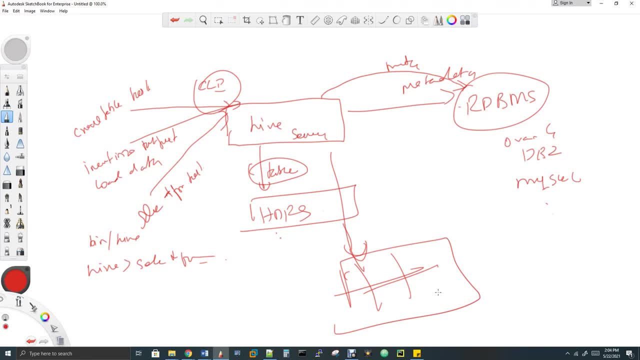 case where the metadata will store. i will tell you that. so you install hive only. okay, i will just go here. so whenever you download hive, right, you installed hive. so when there is no separate rdbms available in your, in your installation, in your machine, then what hive will do? hive itself will. 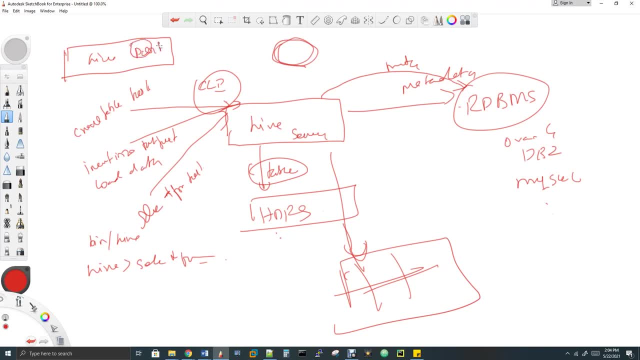 have an embedded rdbms called derby. derby is an embedded. it is an embedded rdbms called derby. derby. internally have have its own rdbms to store the metadata information of hive. we call that. so this will come along with your download and install itself. you don't want to do anything special here. 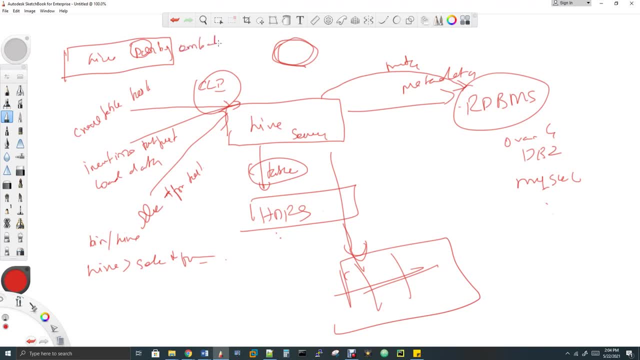 so we call this as embedded. embedded- forgive me for my spelling mistake, so embedded meta store, that means hive itself will have an rdbms called derby. that is very important. it has derby, which you can't change, so it itself has a database derby in which your metadata will be get stored. 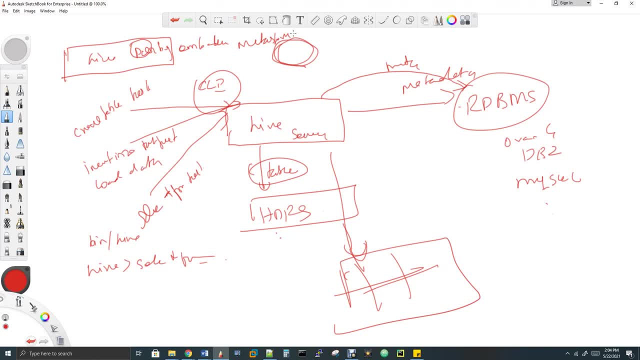 so that you don't want to have a separate rdbms to store the metadata. so we call this as embedded meta store mechanism and we call this as remote meta store- remote meta store. these are important for your understanding as well, as this will be asked in your interview. so now you will get a. 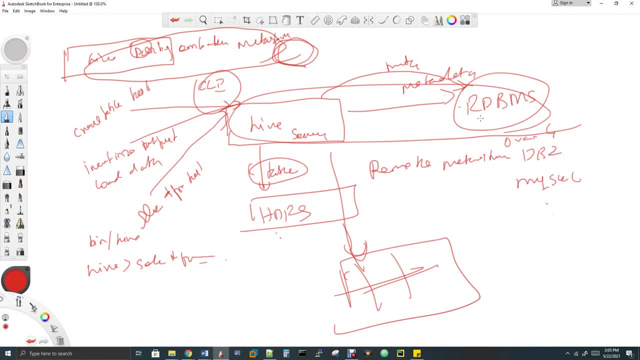 question in your mind. so in that case, why should i have to go for this remote meta store? hive itself has a derby to store the metadata, right? it internally has its own rdbms to store the metadata. then we can go ahead with this itself, right? so we call this as embedded meta store. 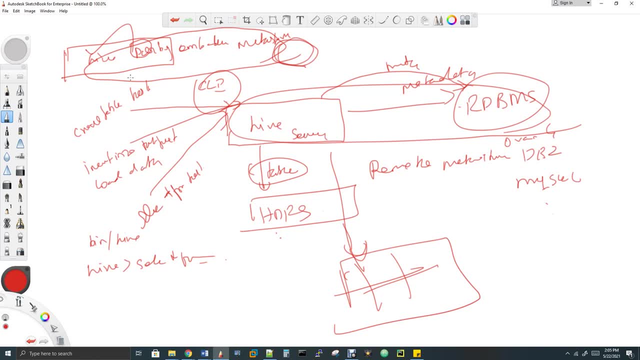 in the real time. in real time, people will not use embedded meta store. they will go for remote meta store. that means they will use a separate instance to store the metadata. i will tell you the difference. i will tell you the drawback of embedded meta store. now imagine you have cluster. 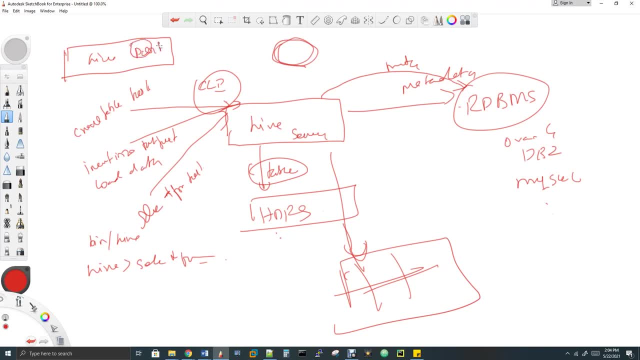 have an embedded rdbms called derby. derby is an embedded. it is an embedded rdbms called derby. derby. internally have have its own rdbms to store the metadata information of hive. we call that. so this will come along with your download and install itself. you don't want to do anything special here. 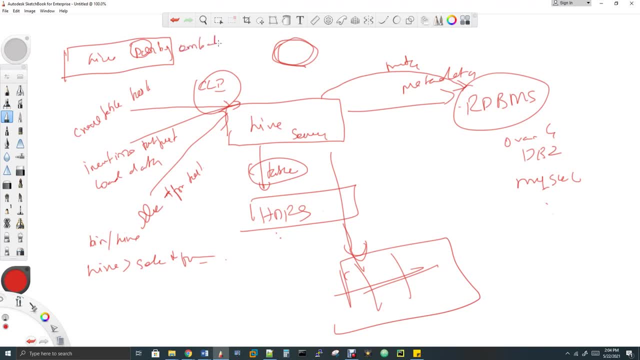 so we call this as embedded. embedded- forgive me for my spelling mistake, so embedded meta store, that means hive itself will have an rdbms called derby. that is very important. it has derby, which you can't change, so it itself has a database derby in which your metadata will be get stored. 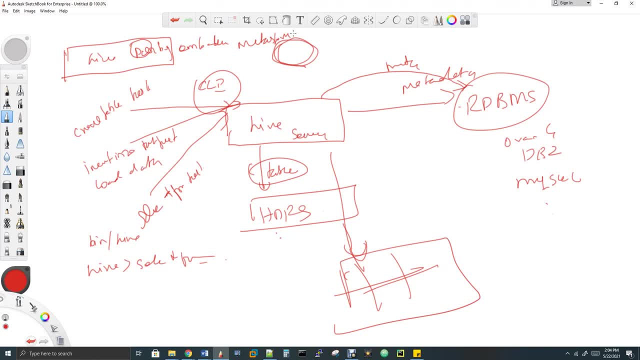 so that you don't want to have a separate rdbms to store the metadata. so we call this as embedded meta store mechanism and we call this as remote meta store- remote meta store. these are important for your understanding as well, as this will be asked in your interview. so now you will get a. 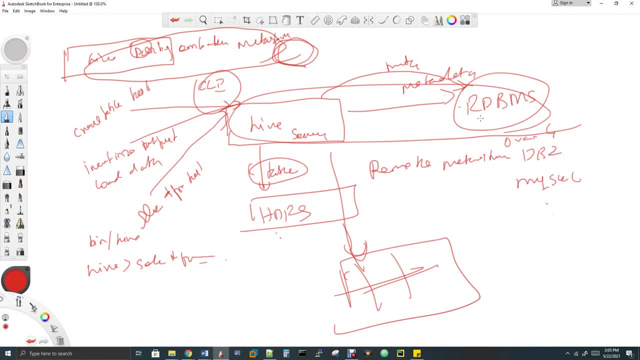 question in your mind. so in that case, why should i have to go for this remote meta store? hive itself has a derby to store the metadata right. it internally has its own rdbms to store the metadata. then we can go ahead with this itself right now. so we will go ahead and install hive. 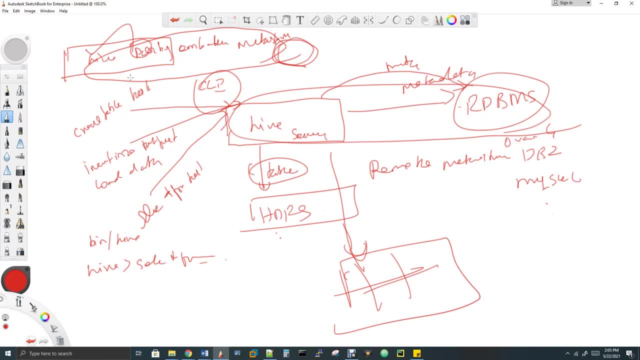 in the real time. in real time, people will not use embedded meta store. they will go for remote meta store. that means they will use a separate instance to store the metadata. i will tell you the difference. i will tell you the drawback of embedded meta store. now imagine you have cluster. 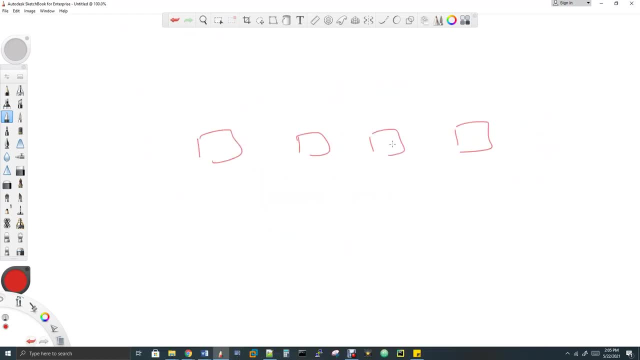 you have four nodes hadoop has installed. so this is four node hadoop cluster. now you install hive in all these node. okay, you download and install hive in all these node and you are not using remote meta store. you are trying to use the embedded meta store that comes with hive itself. 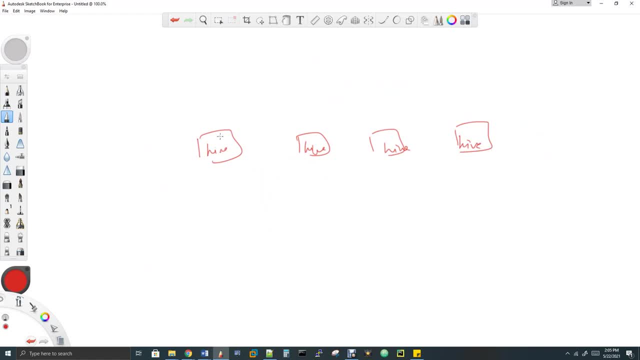 rdbms. that comes with hive itself and that means there will be a derby database here here, here, here, each machine will have its own derby, because in each machine you are installing hive right, so for every hive installation the embedded database will come along with it. now imagine now you are sending and create table request and the request. 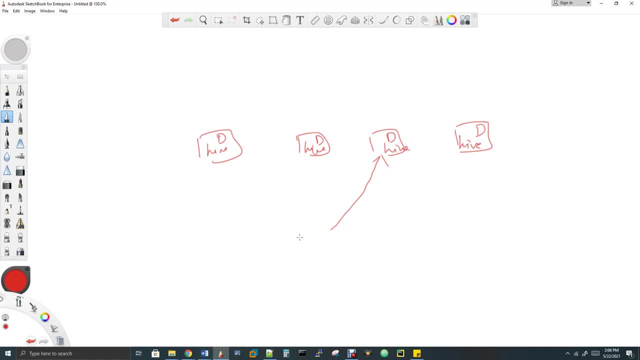 uh, goes to randomly to one node. okay, it goes to third node. create test table test. okay, table test. now what, after receiving the request, what this high will do? this high will store the test. so this tables metadata information in its own derby database, which is an embedded one. 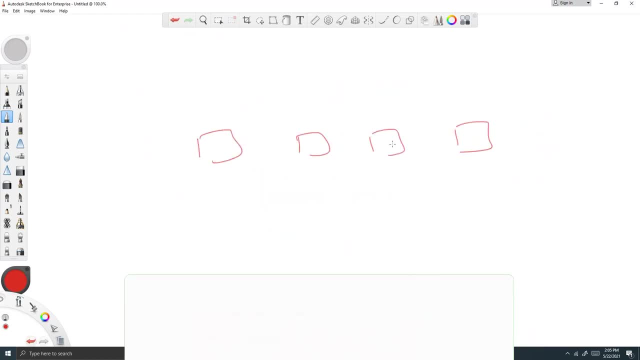 you have four nodes hadoop has installed. so this is four node hadoop cluster. now you install hive in all these node. okay, you download and install hive in all these node and you are not using remote meta store. you are trying to use the embedded meta store that comes with hive itself. 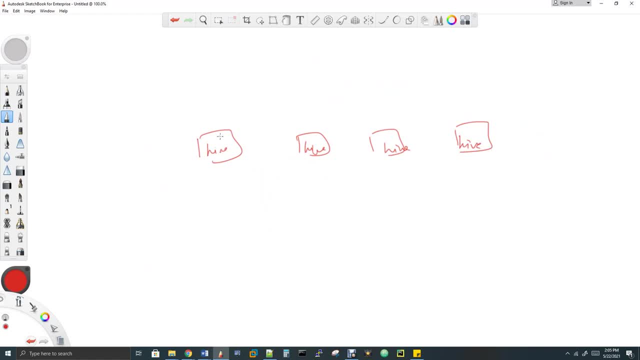 and that means there will be a derby database here, here, here, here each machine will have its own derby, because in each machine you are installing hive right, so for every hive installation the embedded database will come along with it. now imagine now you are sending and create table request and the 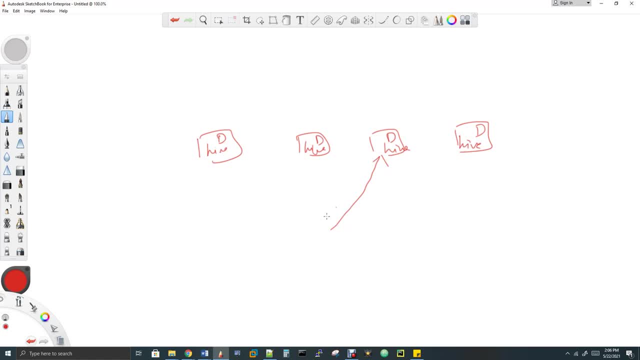 request. uh goes to randomly to one node. okay, it goes to third node. create test table test. okay, table test. now what, after receiving the request, what this high will do? this high will store this, the test. so this tables metadata information in its own derby database, which is an embedded one. 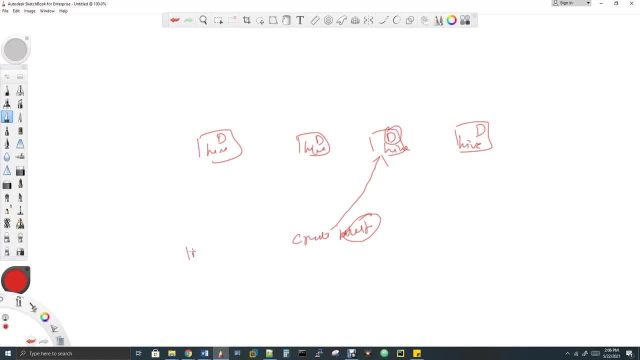 okay. so now there is an another request that you are sending for insert. insert into test, so that request goes to first node. okay, now, after receiving this request, what i will do? it will check whether this test table available in the meta store of derby in first missions hive. so this test table. 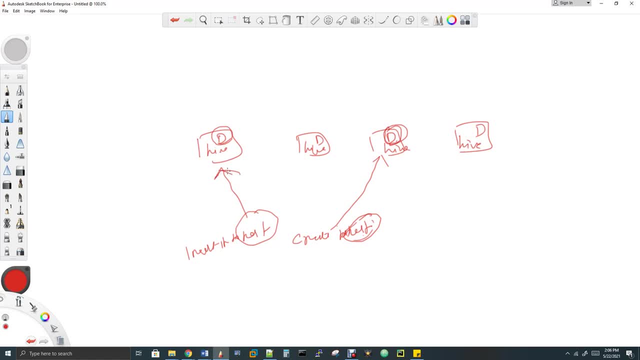 but your insert request goes to first node means it will say table not found. now you understood the problem of why we are not having embedded in the real time. so each node high will have its own metadata. so you can't do a distributed request. so there should be an one place where all the metadata. 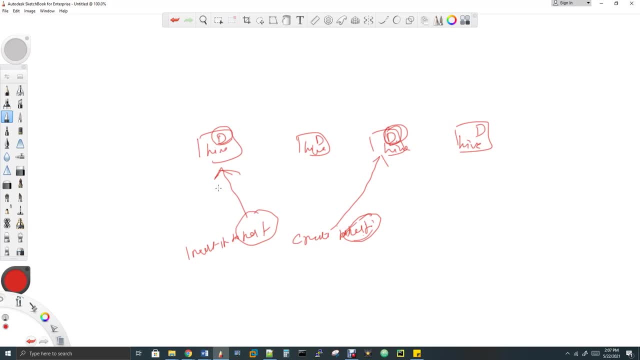 should store there. so all these four hives should refer that and that is where we are going for remote meta store. we are not going for embedded meta store. so now you in in the same cluster, you install like one more node, mysql, so where you can configure. so there is a configuration file. 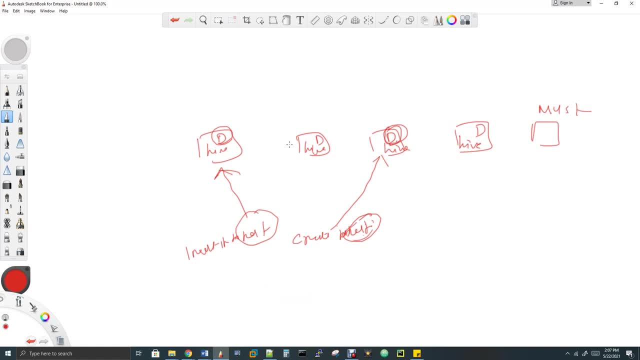 in your hive where you can say like, use remote metastore, not embedded. this is what i have showed in my hive installation video. you can refer that there is a configuration file, so uh. so in all these hive configuration file i will say: use this mysql node, the fifth node, so now the embedded. 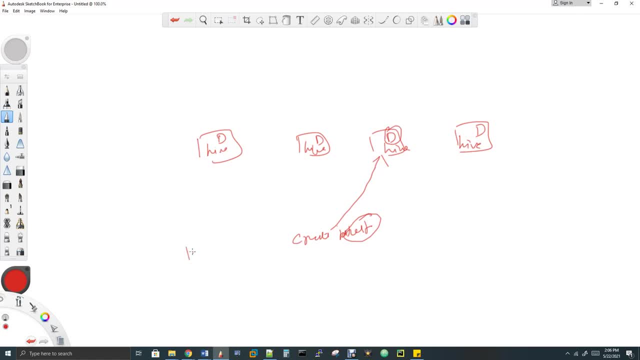 okay. so now there is an another request that you are sending for insert. insert into test, so that request goes to first node. okay, now, after receiving this request, what i will do? it will check whether this test table available in the meta store of derby in first missions, hive. so 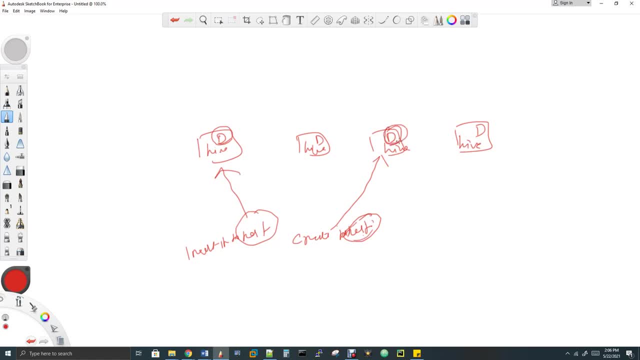 this test table metadata gets stored in third missions. derby right. but your insert request goes to first node means it will say table not found. now you understood the problem of why we are not having embedded in the real time. so each node high will have its own metadata, so you can't do a distributed request. 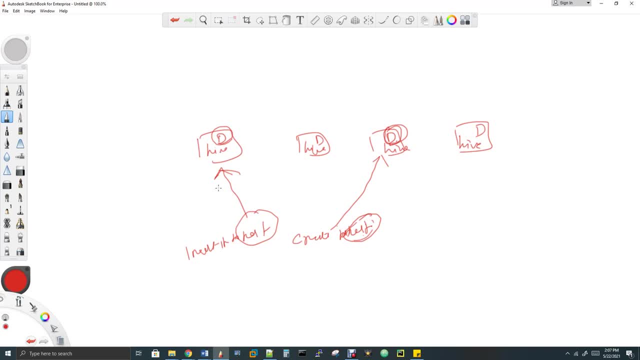 so there should be an one place where all the metadata should store there. so all these four hives should refer that, and that is where we are going for remote meta store. we are not going for embedded meta store. so now you in in the same cluster, you can install like one more. 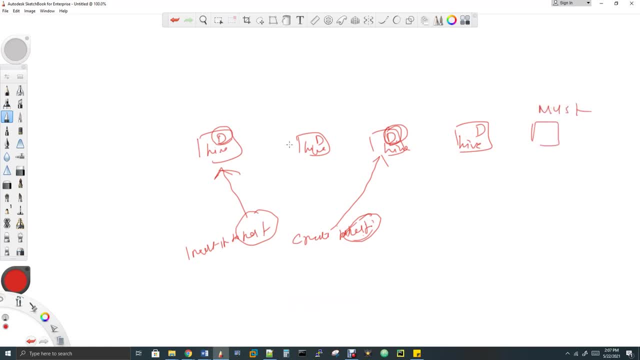 node mysql, so where you can configure. so there is a configuration file in your hive where you can say, like use remote meta store, not embedded. this is what i have showed in my hive installation video. you can refer that there is a configuration file. so so in all these five configuration file i 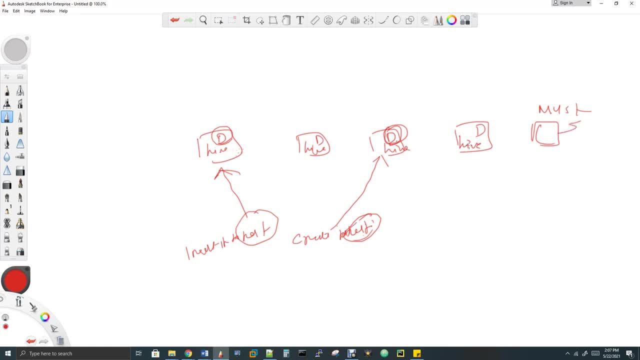 will say: use this mysql node, the fifth node. so now the embedded derby will remove automatically. so when there is a remote or database there it will not use the derby. now, when you send a create table request to third node of hive, this high will store the metadata of test table here. here the metadata: 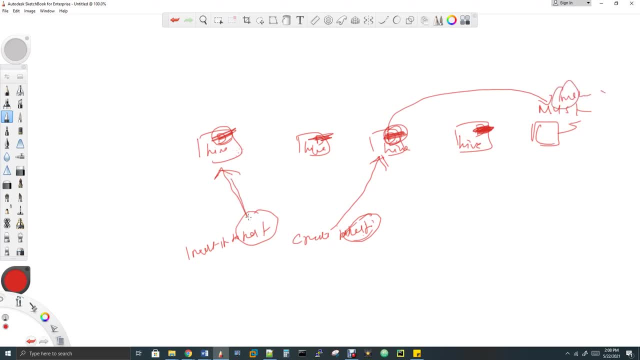 will be get stored. now you are sending an interest. sorry, insert request to first hive node now. now again i will search for the test table, whether present or not here, so it is commonly accessed by all nodes. so now test table metadata is already stored right, so now your table will be successfully. 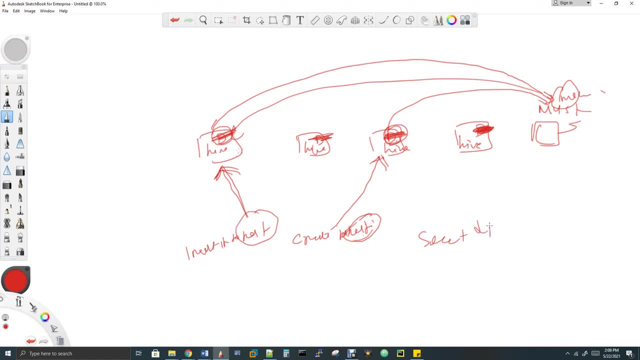 stored. now again you can run a select query. the select star from test request goes to four node. again this i will refer this common metadata and this i will show you the table. so this is why we are not going for embedded, we are going for remote. so what is the use of embedded? 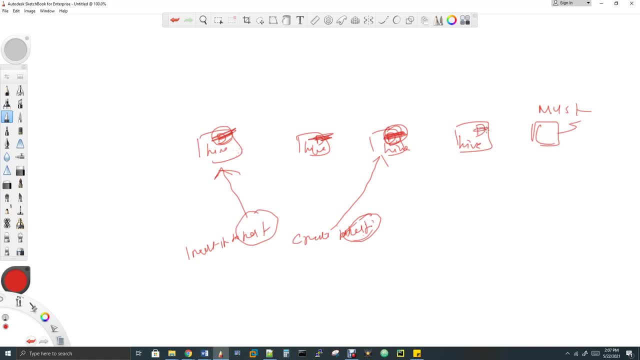 derby will remove automatically. so when there is a remote database there it will not use the derby. now, when you send a create table request to third node of hive, this hive will store the metadata of test table here. here the metadata will be get stored. now you are sending an interest, sorry. 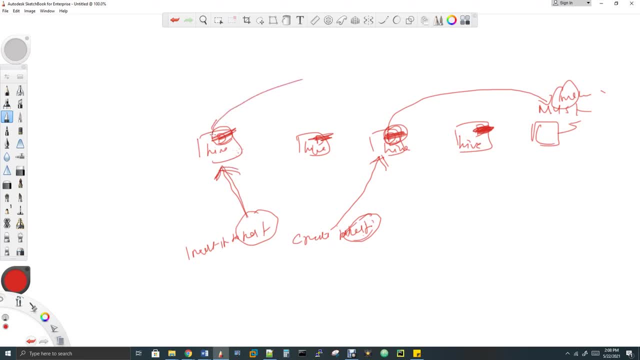 insert request to first hive node. now, now again, hive will search for the test table, whether present or not here, so it is commonly accessed by all nodes. so now test table metadata is already stored. right, so now your table will be successfully stored. now again you can run a select query. the 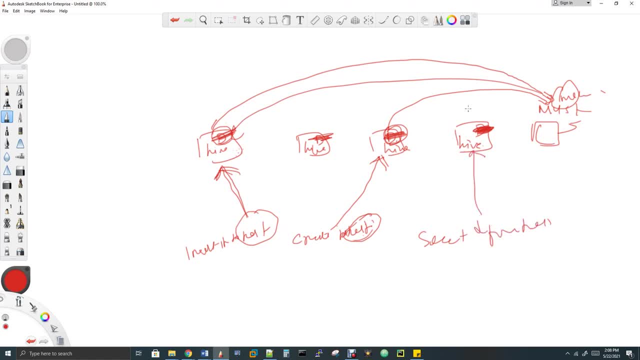 select star from test request goes to fourth node. again, this hive will refer this common metadata and this hive will show you the table. so this is why we are not going for embedded, we are going for remote. so what is the use of embedded derby then? so in a single node machine you are, you just need to install hive. 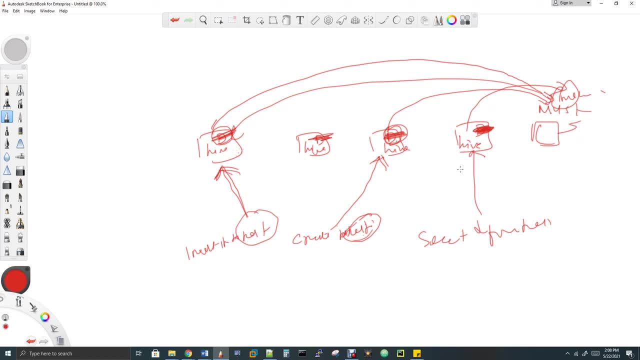 just for practice purpose. you can go with embedded. you don't want to sit and install separately rdbms to store the metadata just in a single node. it's not required, but it's recommended even in single node. it is recommended so that you will come to know what it is actually. 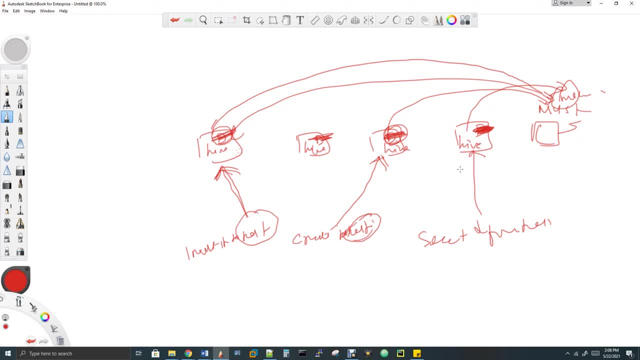 so that is why i added the, the mysql part as a remote metastore part in my hive installation video. you can refer that and this is what hive architecture is all about. the internals are all about. so here only with the cla you can connect or we have any other mode of communication to. 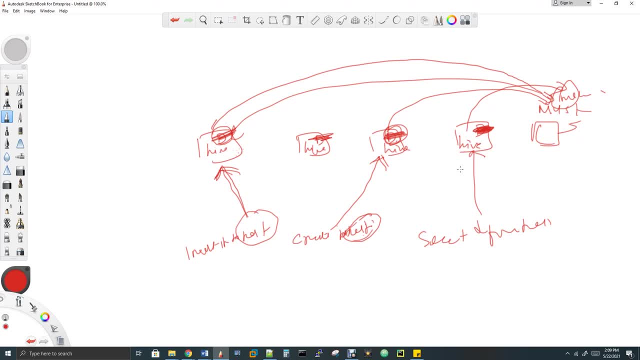 connect with hive. you can do jdbc connection also, okay. so jdbc connection is something. you write a program to connect with hive. you are building a web ui to connect with hive. then we need to go for jdbc, so jdbc is also possible. again, the request response will happen in. 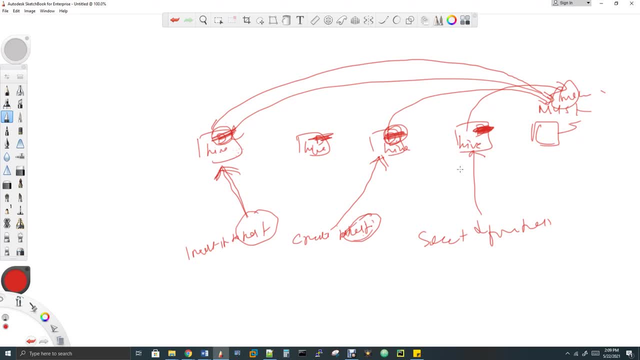 the same order, the same way, how i explained it to you. okay, so the so hive end of day. hive runs with the three engines, so by default, hive runs on map reduce engine. there is another engine called the taste and there is one more called spark, so you can run hive on top of. 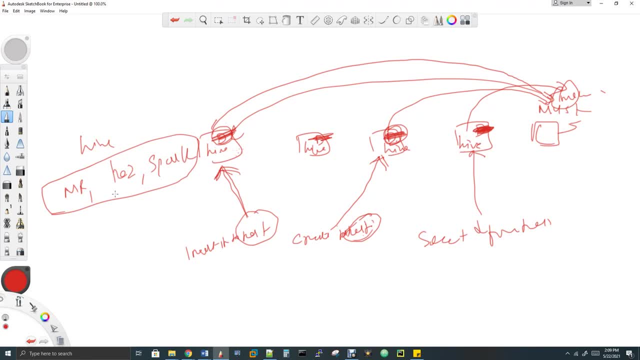 these three engines. end of day your data will be get stored in a distributed file system like hdfs and even the. in amazon there is a object stored called s3 that is also similar to hdfs. so even hive can be used with s3. so you can run hive on top of these three engines and 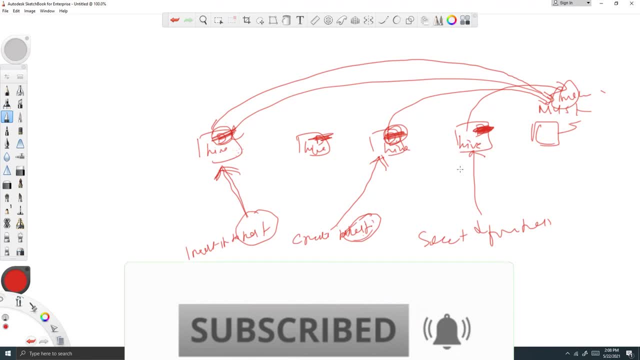 derby then. so in a single node machine you are. you just need to install hive, just for practice purpose. you can go with embedded. you don't want to sit and install separately or the bms to store the metadata. just in a single node. it's not required but it's recommended even in single. 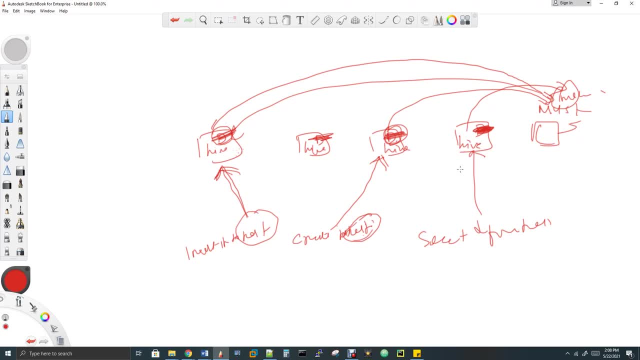 node. it is recommended so that you will come to know what it is actually. so that is why i added the my sql part as a remote metastore part in my hive installation video. you can refer that. and this is what hive architecture is all about, the internals are all about. so here, uh, only with the cla you can. 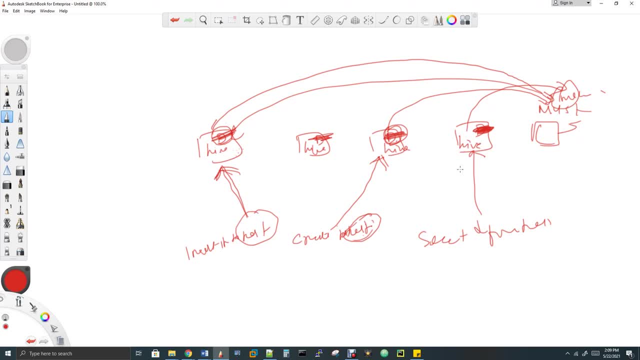 connect or we have any other mode of communication to connect with hive. you can do jdbc connection also. okay, so jdbc connection is something. you write a program to connect with hive. you are building a web ui to connect with hive. then we need to go for jdbc, so jdbc is also possible. 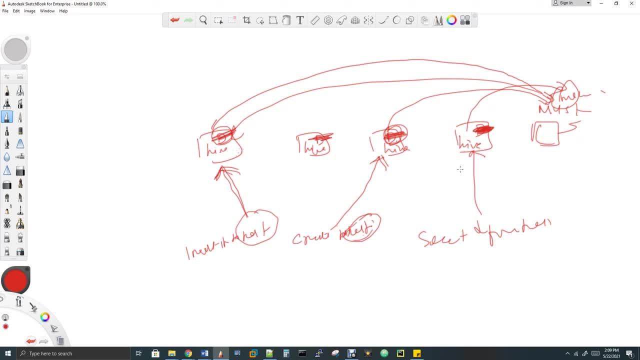 again. the request response will happen in the same order, the same way how i explained it to you. okay, so the so hive end of day. hive runs with the three engines, so by default hive runs on map reduce engine. there is another engine called the taste and there is one more. 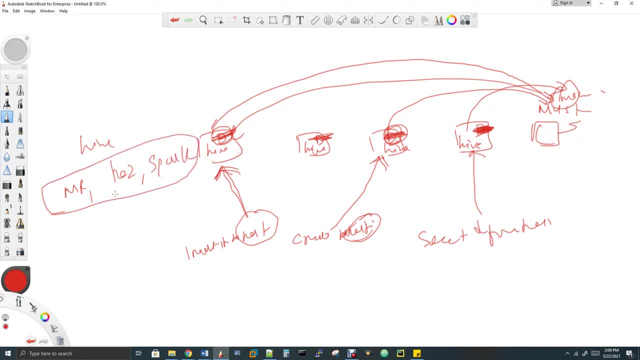 called spark, so you can run hive on top of these three engines. end of day, your data will be get stored in a distributed file system like hdfs and even the. in amazon there is a object stored called s3 that is also similar to hdfs, so even hive can be used with s3 also. okay, so not only hdfs. 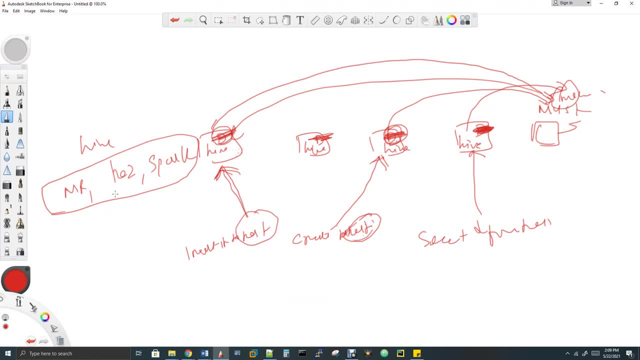 it can be used with s3. so if you are not aware of s3, don't worry. you don't want to get confused for now. so hdfs is aware. place hive will store the data. metadata will be get stored in an rdbms. okay, either embedded or remote rdbms. that's it okay. so thanks for watching data. 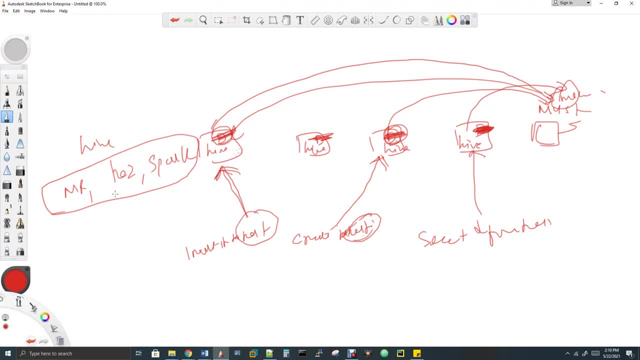 engineering. as i told you already, i have given complete hadoop spark hive in a category of playlist in the description box. you can refer that for all the videos. okay, so, and also like my instagram id and my uh email id is given there, you, if you want to. 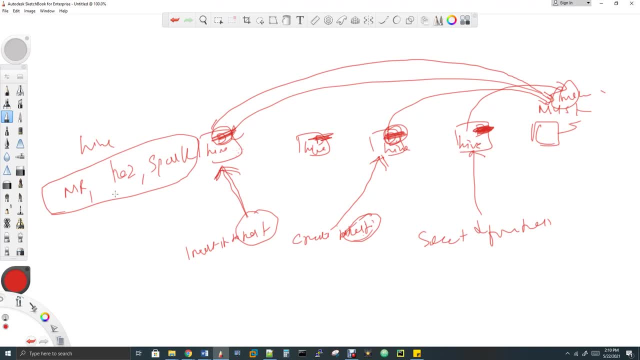 contact you can contact and please do share with your colleagues and friends and please share my link in your linkedin. that will be very helpful for me and thanks for watching data engineering.